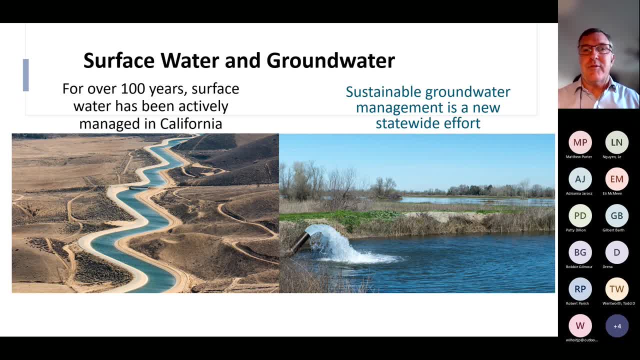 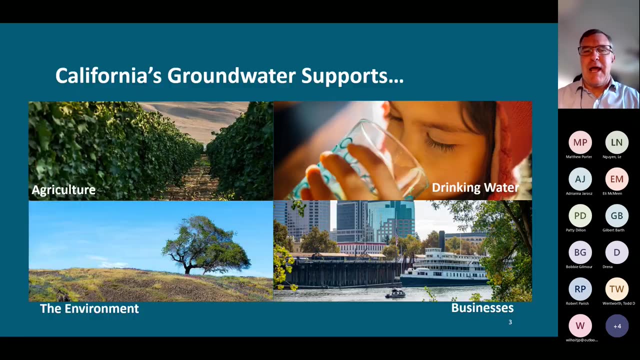 So SGMA came about out of necessity. We saw a lot of dry wells and a lot of impacts, So the legislature took action in 2014 and enacted The Sustainable Groundwater Management Act, also known as SGMA. So you know, for Californians, many people don't have a grasp of what California or what groundwater is. 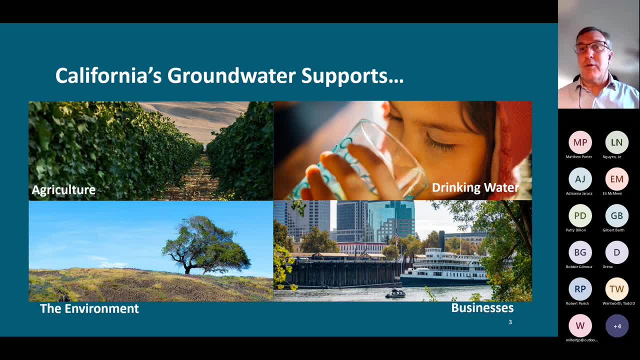 And these are largely. we're focused on our alluvial groundwater basins. in the state which we have, 515.. I'll talk about that a little bit more, But in general, our groundwater supports our drinking water systems, our environment, our industrial business practices, including agriculture. one of the largest in the world. 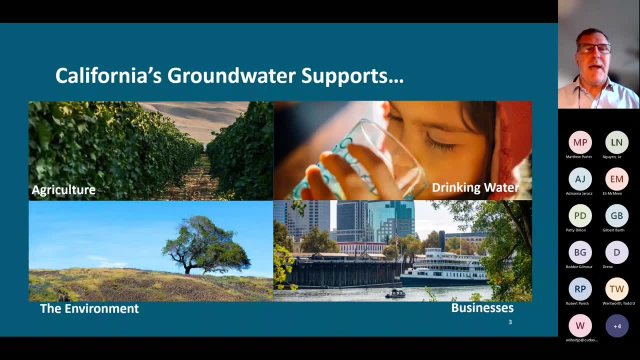 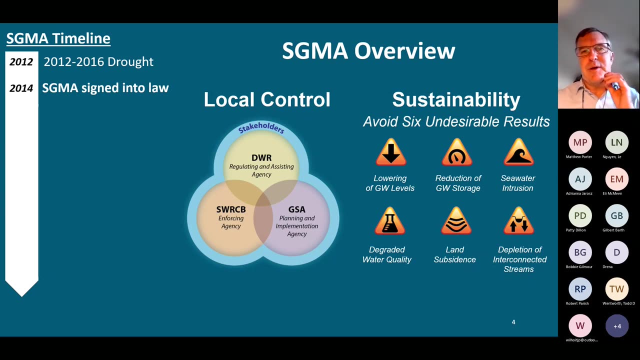 And so it's very imperative that we start to manage these resources so we don't continue to see the impacts that we have been been observing for the last several decades. So a quick run through in the timeline of SGMA, but this is an important slide. 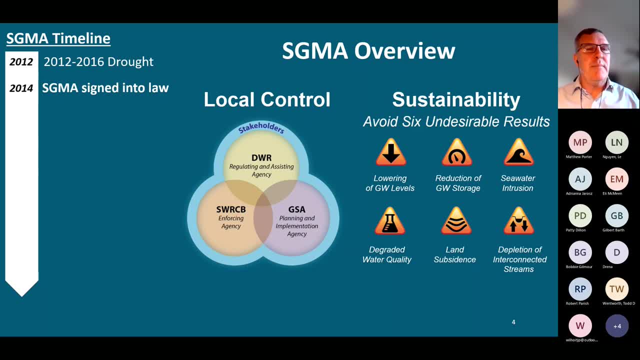 I want to spend a couple of times on a little bit of time on just to describe what the major building blocks are of SGMA. So again, I mentioned in 2014,. the law was signed, The bill was signed, The bill was signed into law and we began implementing SGMA. at that point, 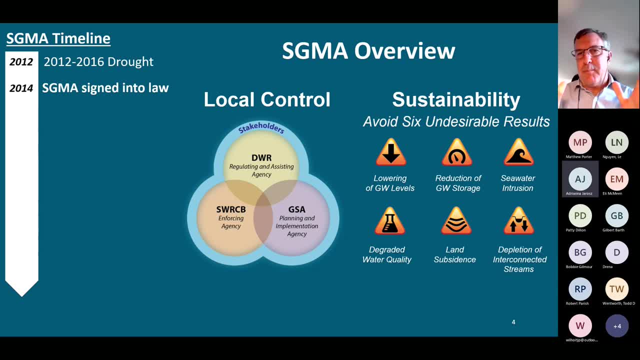 So who does it affect? One of the primary functions here is that SGMA relies upon local agencies to define sustainability locally, based upon consideration of the beneficial uses and users in the basin and how groundwater is utilized and what those impacts could be. So there are four main groups of people here that are represented. 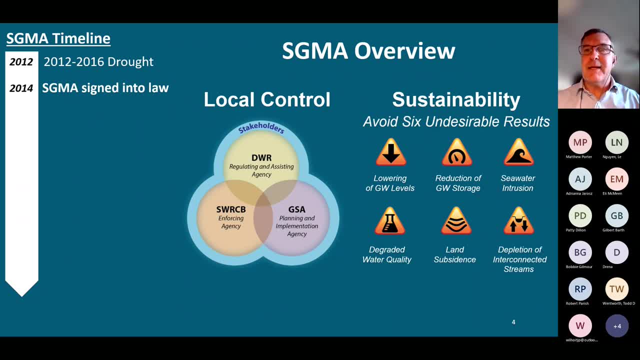 The stakeholders, These are our beneficial uses and users. These are the people in the basins, These are the people utilizing groundwater and it's imperative that the local agencies engage with them to define what sustainable conditions are in the basin. And so then then we have the local agencies. the local agencies under SGMA were required to develop groundwater sustainability agencies, so brand-new government entity to manage groundwater, moving forward. 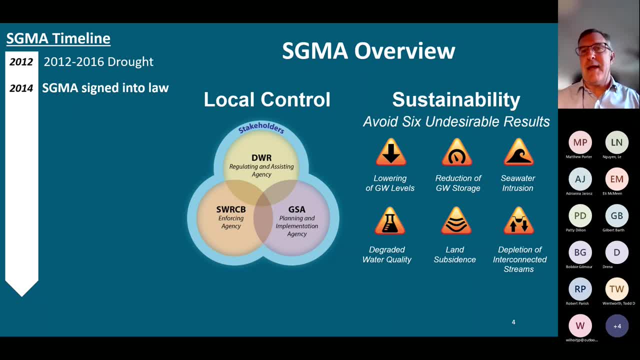 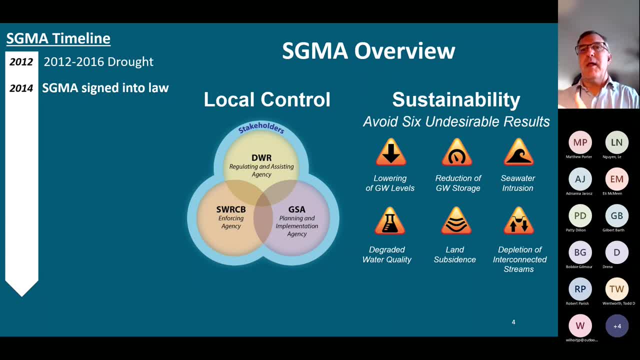 with, But these water managers were largely providing water supply. Now they're being tasked with managing the groundwater system. So there's a big learning curve and they've been working diligently to get over that curve and get SGMA implemented. Then there's the Department of Water. 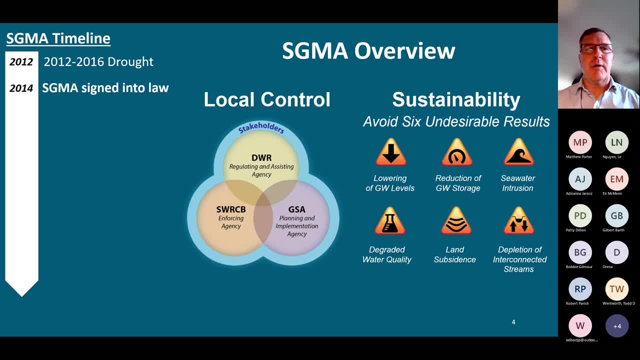 Resources. That's DWR. That's the agency that I work for. Our responsibility is twofold: It's a regulatory responsibility as well as an assistance function. So the regulatory responsibilities include the review of the groundwater sustainability plans and making sure that folks. 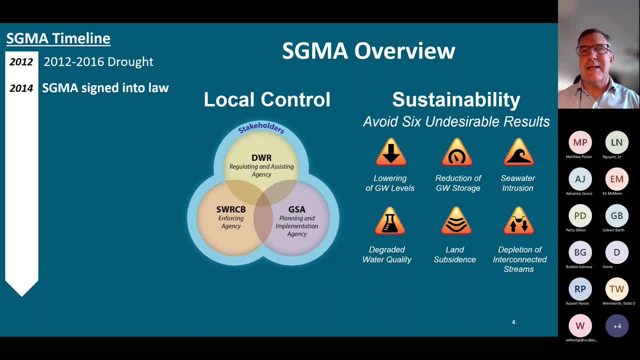 are moving in an adequate fashion towards their sustainability goals. And then we also have the State Water Resource Control Board. State Water Resource Control Board in California is responsible for administering our surface water rights system. So they are integral to, you know, really allocating the surface waters and making sure that they are being managed. So they are being 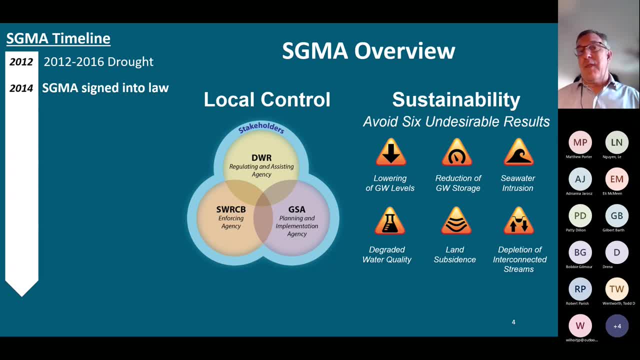 put to a beneficial use across the state. They serve as a backstop. Should the department determine that local agencies aren't making adequate progress or failed to develop a plan, they can step in and help manage the basin while the local agencies correct their deficiencies or get things in line. 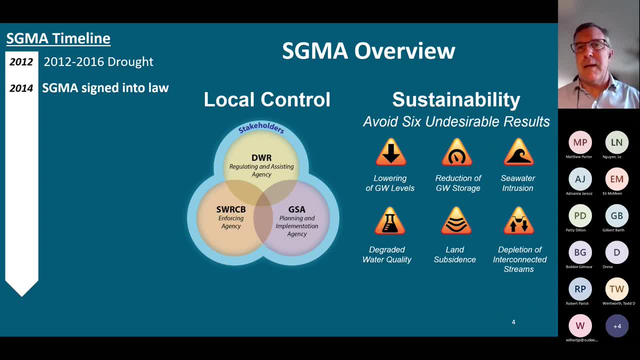 and then keep moving, returning the oversight back to the department once things are righted. So that's the two blocks in terms of who the players are in SGMA. Now, what is sustainability under SGMA? This is a unique approach to defining sustainability. So sustainability under SGMA is: 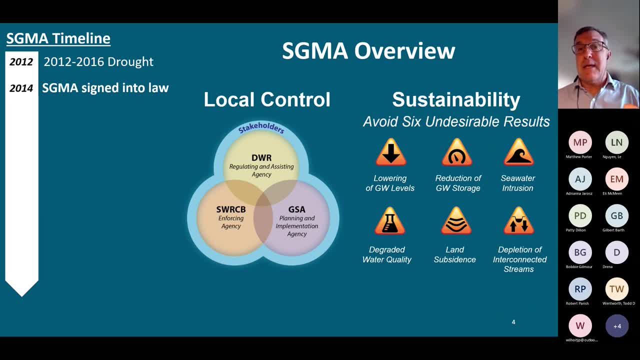 defined as operating to a sustainable yield. So we can think about a water budget for a given basin. There's the inputs, the outputs, Obviously, if you're taking more out, then it's coming in. you're depleting that basin. 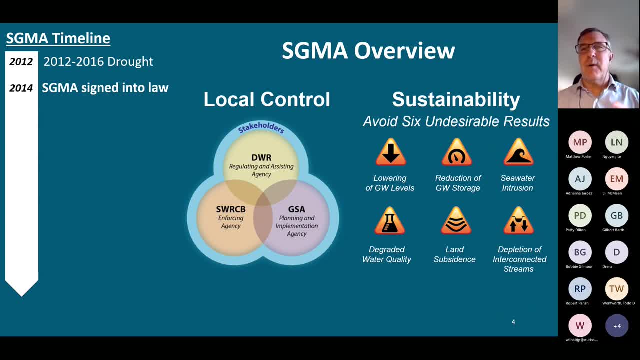 That's one step, But layered on top of this is the avoidance of undesirable results, And this is where the local control comes in. We really want local agencies to engage with the, with the beneficial uses and users of these, of these waters within their basins, to define what is a significant and 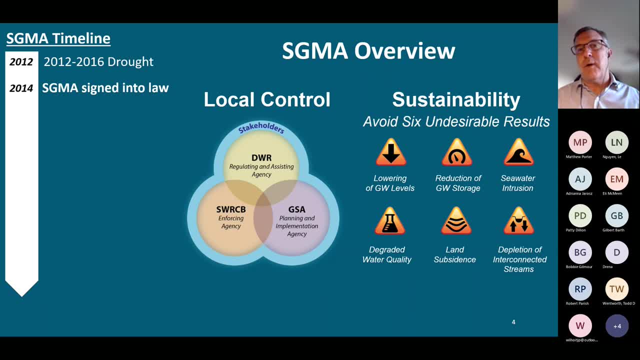 unreasonable impact to the basin that they want to avoid. So not only operating to a yield, but also avoiding these impacts. And those impacts include chronic lowering of groundwater levels, significant reductions of groundwater storage, seawater intrusion, degraded water quality, land subsidence and, probably the most technically challenging one, the depletion of interconnected 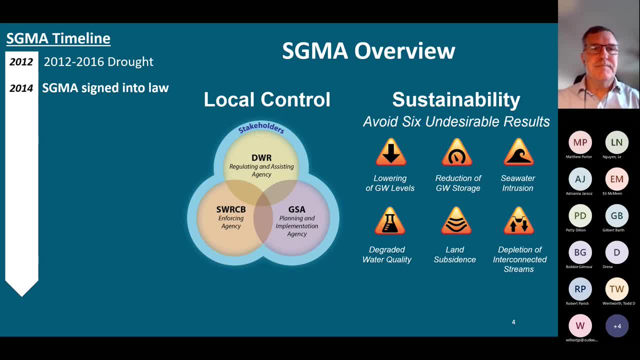 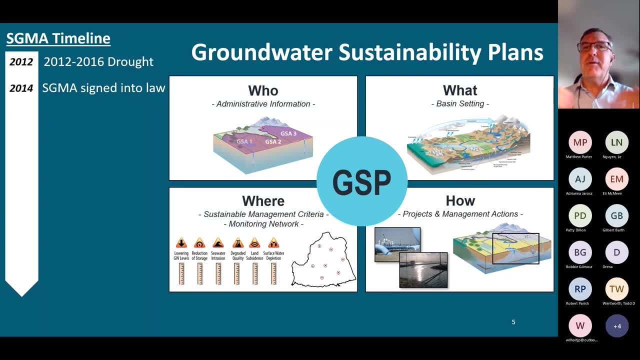 surface waters and streams. So what's in a groundwater sustainability plan? So we've developed regulations to help local agencies understand what is required to be defined in these and provide information so that we can see that they have a clear plan towards meeting their objectives, which is operating to the sustainable yield and avoiding 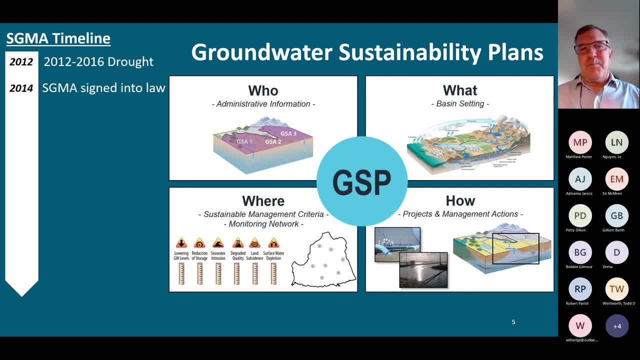 those undesirable results. So basic sections. Who is this? Who is in the basin, Who are the beneficial uses and users, who are the local agencies that are part of this, Who are the counties and cities and all the people that are reliant upon? 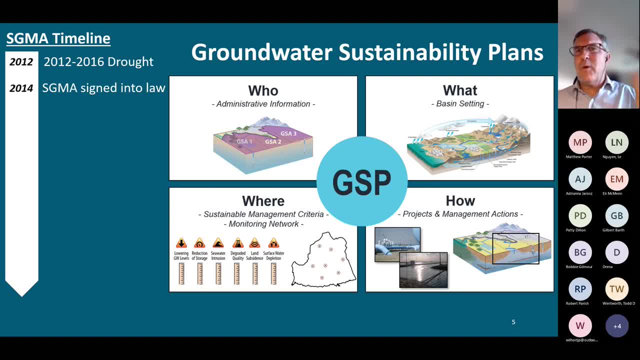 the groundwater resources in the state, The what. What's going on in the basin in terms of groundwater? What are the conditions? What's the geology? What's the land usage, построing of the verschiedenen� land use practices? what is your water budget for this basin? how, what are the inputs and outputs? 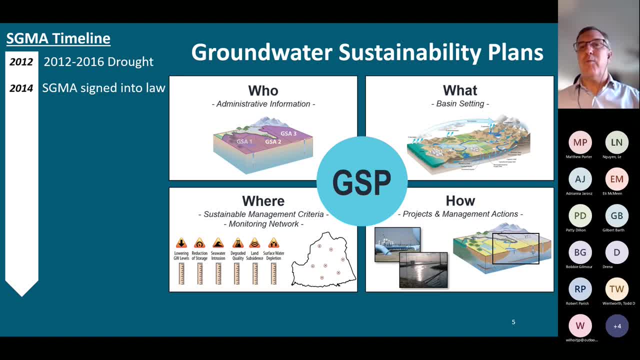 and, as you can imagine, in california we have a lot of water coming into and out of basins through surface water projects and moving waters through canals and those kinds of things, taking water from where it is up north for us to the south where we have most of our beneficial users. 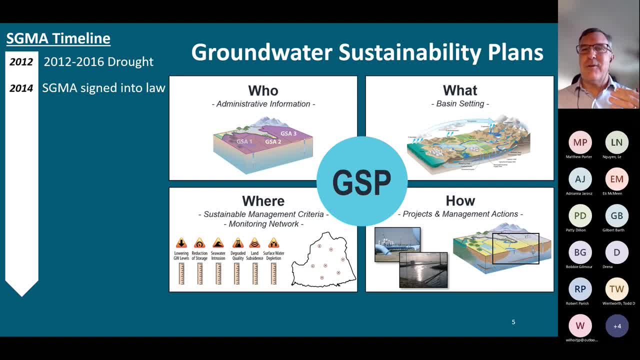 so it's a very complex system in that sense that we have to not only account for what's going on physically and under natural conditions within the basin, but then also what is managed and imported and out and and exported from the basins. then we have um the where aspect, how are, how are? 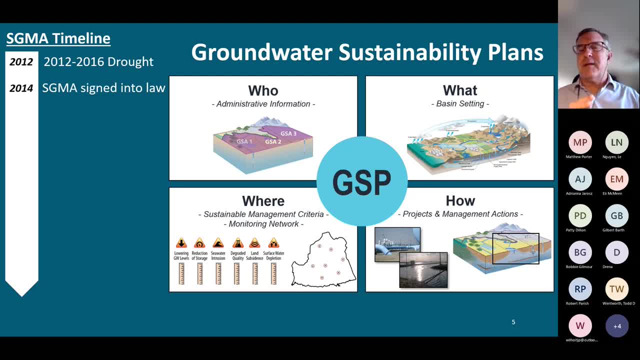 the local agencies, quantifying and demonstrating to all the beneficial uses and users and the department how they are avoiding these undesirable results. so this required the establishment of several metrics, quantifiable metrics, um, the first of which is the minimum threshold, so below which um you might start to see adverse conditions occur and and potentially undesirable. 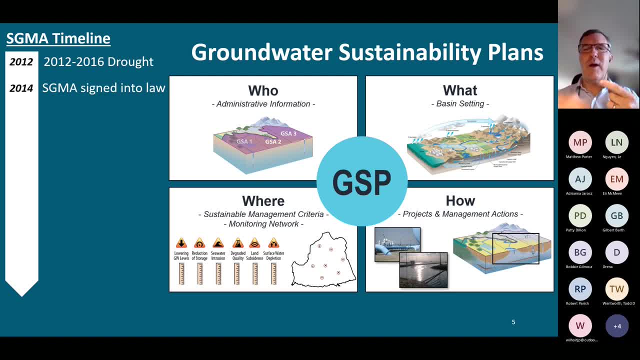 results and then measurable objective. what's your target? where are you going to create a target for you to achieve? so, rather than manage to scarcity, we're going to push it towards managing, towards abundance. we want to have this buffer, if you will, of water well above the threshold below which you. 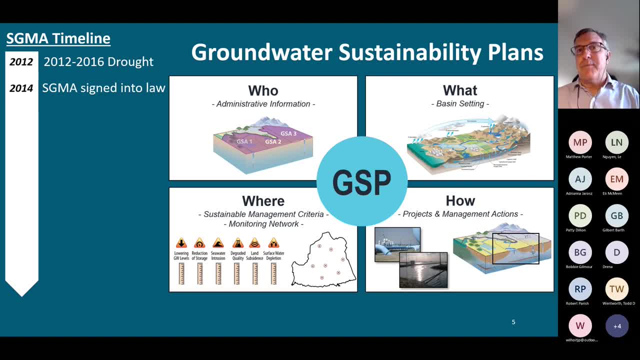 could be having bad things happen, and then how. this is the big ticket item. many of these basins are in overdraft and they are looking at how can they implement projects and management actions to balance that water budget and avoid the undesirable results so effectively. there's two knobs: there's a supply knob and there's a demand knob. most agencies don't even. 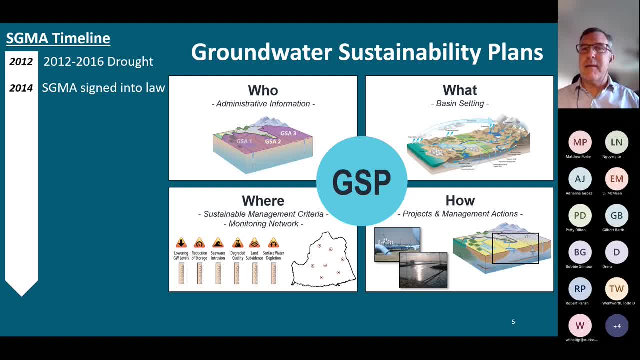 want to look at the demand knob. they want to add more supply so they can maintain their current you know uh, economies and and social structures. so we're basically talking about agriculture in in, in these basins where sigma is being applied. demand reduction means the reduction of of agricultural footprint, largely um in and amongst. 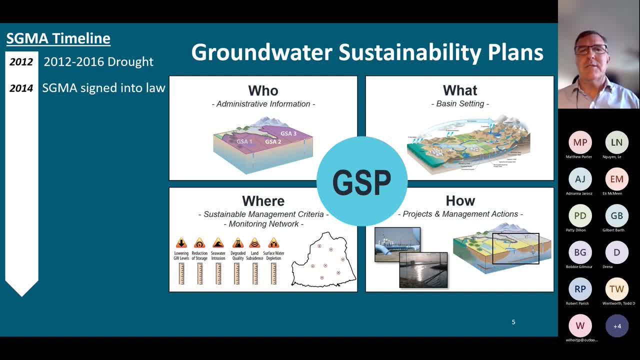 uh, conservation efforts and and those kinds of things. so it's really challenging for local agencies to say: this is a great idea. we need to reduce. reduce the demand, which means stopping pumping early projections for the next few years. so we're going to be looking at some of these things as we move forward. 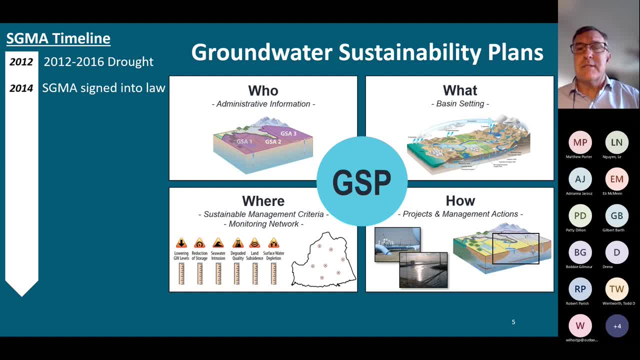 i'm going to talk about the impact to the agricultural community, where anywhere from three quarters of a million to a million acres of agricultural lands may need to be brought out of production. that takes a significant hit in terms of the food and fiber produced for the nation, not 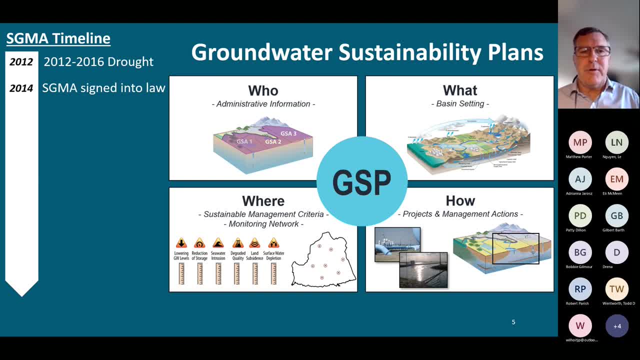 just california. so these are, these are impacting issues that that affect more than just california and uh, so just want to flag that for you. these are challenging issues that we're trying to work extent possible. So again, I highlighted we had a rulemaking process. We developed both a set of 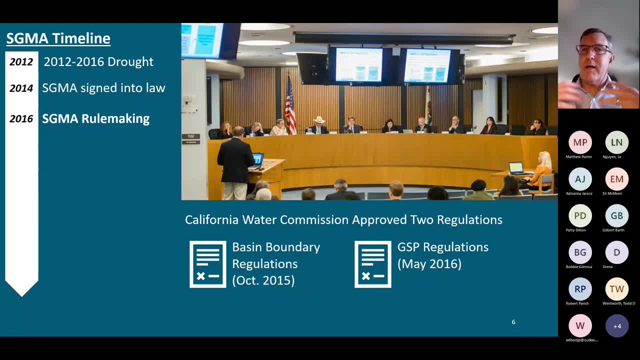 regulations for basin boundary modifications. So we want to rely upon the best available science, And this is a great opportunity for local agencies to come forward and say: yeah, DWR, you don't have the best information. Here's some detailed analysis that we've done. 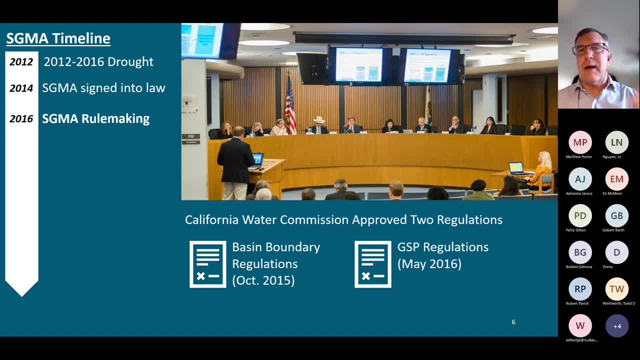 This is how our basin is configured, that we can manage it. So those are out there. We've already had a couple of rounds of those. We're now on hold in that process, just allowing for the groundwater sustainability plans to take effect and start to learn more information, And then we 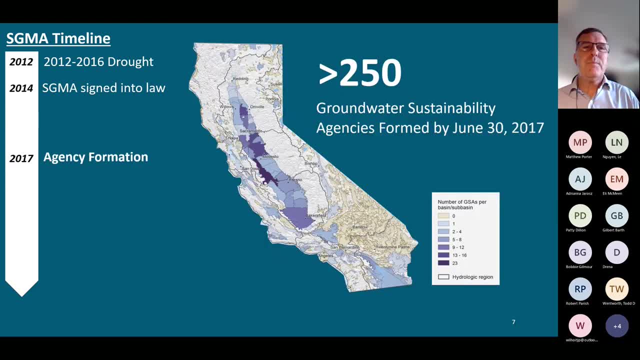 also have the regulations for the groundwater sustainability plans, So I alluded to the groundwater sustainability agencies. We have more than 250 new government agencies now tasked with managing groundwater in a state that hasn't been managed before under a regular transition. So we're now in a state that hasn't been managed before under a regular transition. 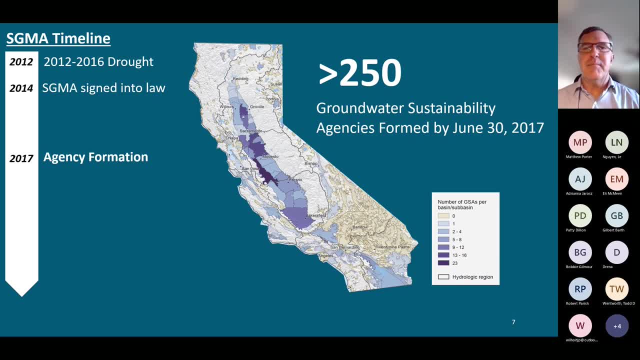 So this is a big task and a big move, And I'll just say that all of the local agencies stepped forward and took this challenge on. So we had 99.9% compliance for this thing And the 0.1% was 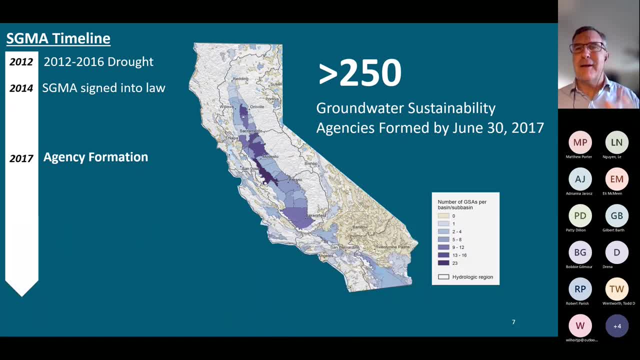 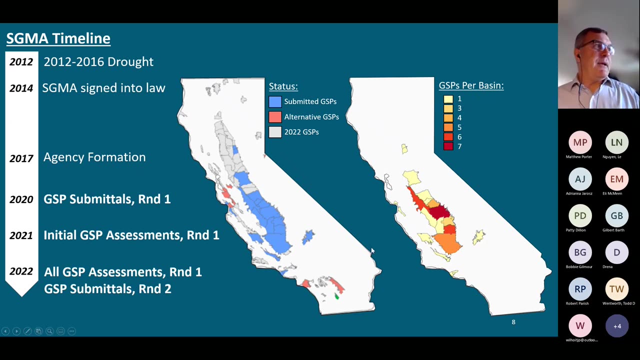 administrative challenges that they were working through, and we resolved those. So we see strong commitment towards implementing this. People recognize the necessity of it, despite it being so challenging to implement. And then where do we see this happening? So we look across the basins. So 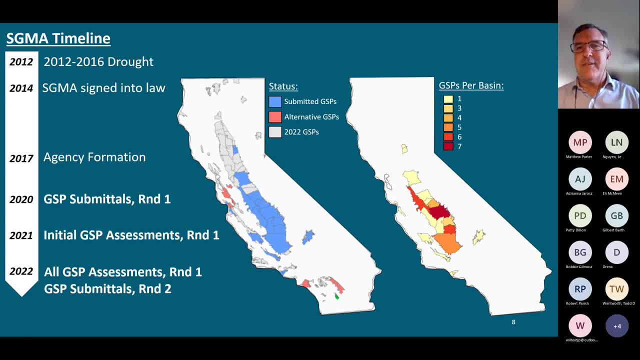 SGMA required a couple of sets of submissions. In 2020, we've identified the critically overdrafted basins. Those basins had to submit their groundwater sustainability plans to us by January of 2020.. All the remaining high and medium priority basins were required to submit. 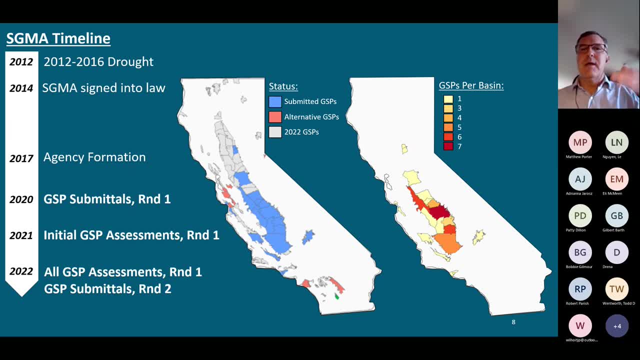 plans in 2020.. And so we're now in a state that hasn't been managed before under a regular transition. So you can see there's a little bit of a staggered effect with the law calling upon the most impacted basins to take action early rather than later. One of the complexities of SGMA is it also. 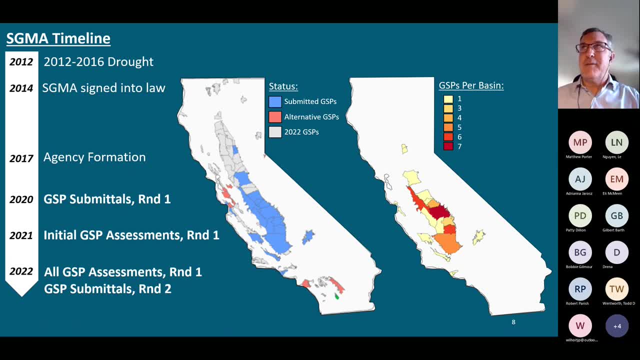 allows for, despite the basin being the base unit of compliance, the area over which we're trying to define sustainability. it also allowed for multiple plans to be submitted for these basins And, as you can imagine, at the local level there's a lot of. 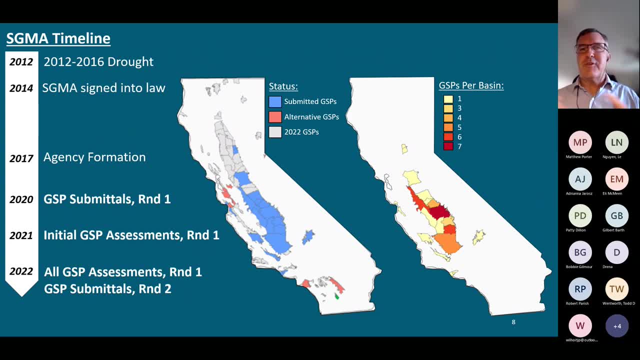 dispute about how things get done, And this creates a lot of challenges for accurately and consistently quantifying our resources and how it's to be managed. So what you can see in the graphic on the right is we have a majority of our critically overdrafted basins submitting. 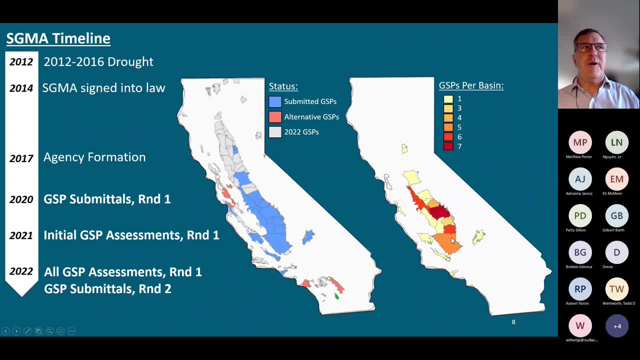 a single plan that covers the basin, but a handful that are submitting multiple plans. Those plans have to be managed under a coordination agreement which clearly defines the methodologies for the quantification of the metrics in the basin. That's a tall order. Most people like to do it their way and not the other guy's way, So it presents a significant 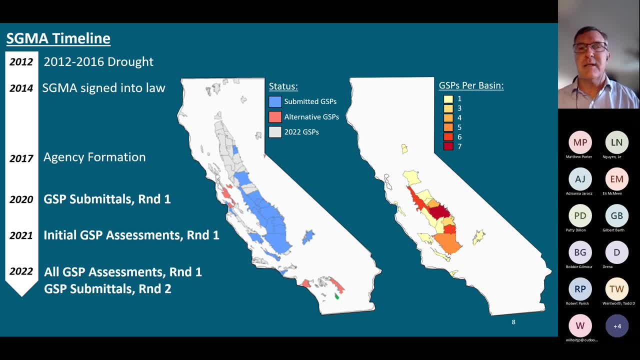 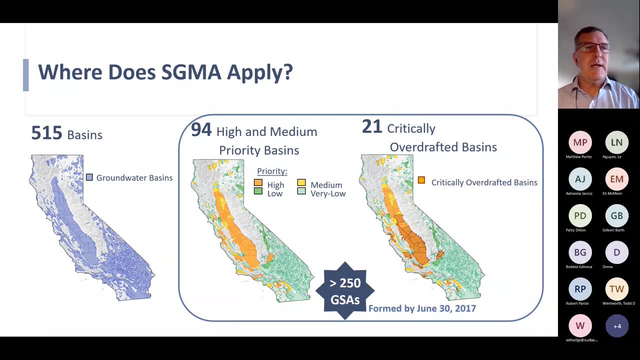 challenge, but most are working through those challenges and taking significant actions. Again, I'll just touch on the basins that we've been working. in The graphic on the left, we've identified 515 discrete alluvial basins within the state. 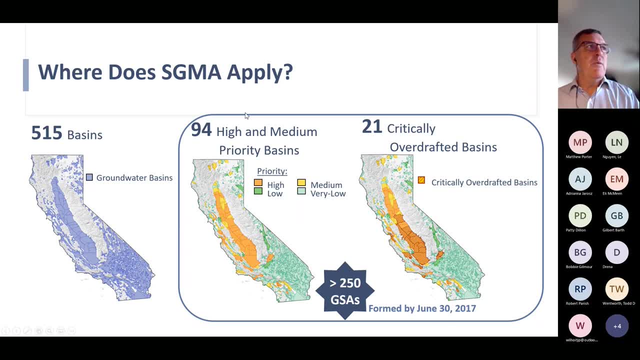 And these are the base unit for compliance under SGMA. We also had to conduct a prioritization process where we identified categories of very low through high for this purpose, And you can see that the middle graphic highlights those in orange and yellow as those that are medium or high priority and are required to. 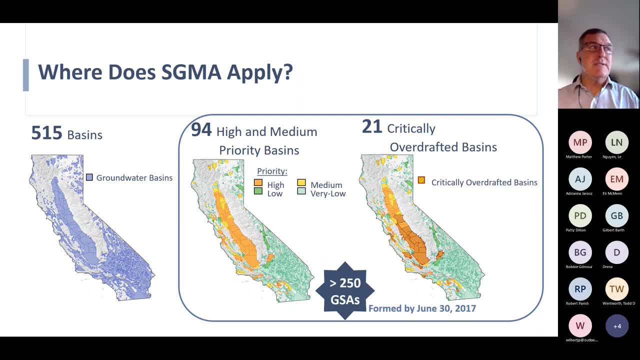 comply with SGMA, Developed GSAs and GSPs. So what does prioritization mean? It's not a reflection of bad water quality conditions. it's a reflection of the dependence on groundwater within that basin. how much is? how important is groundwater to their water water supply portfolio? should it be managed? 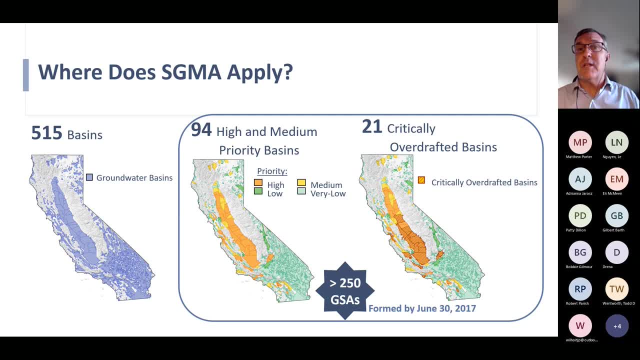 or not. so that's a that's how the prioritization really shuffles out, and there's a pretty significant effort to compile all of this data and information. on top of that, we identified critically overdrafted basins, and these are basins where we have known impacts: chronic groundwater level. 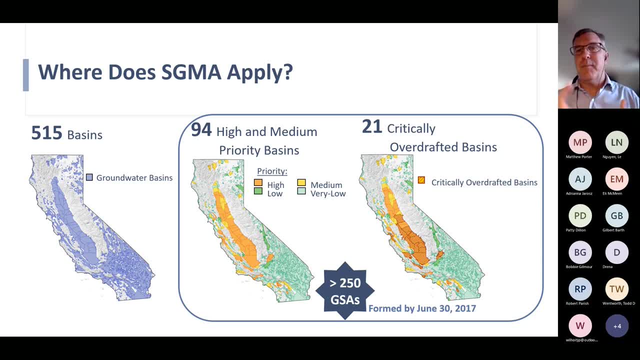 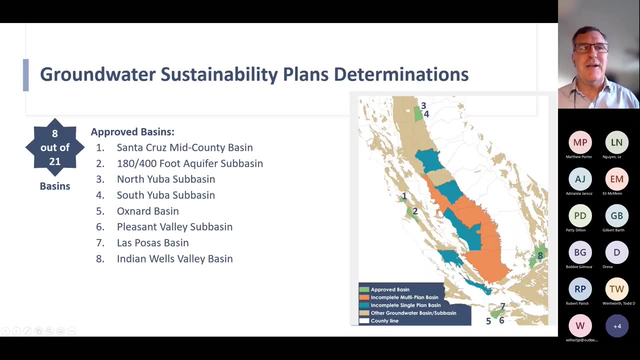 declines, dewatering of water supply, wells, subsidence conditions, sea water intrusion or significant degradation of the water quality within the basin. so those have been flagged for quite some time and are now, you know, got a purposeful meaning once SGMA was created. as to how to move forward, okay, so where do we stand? we have currently received 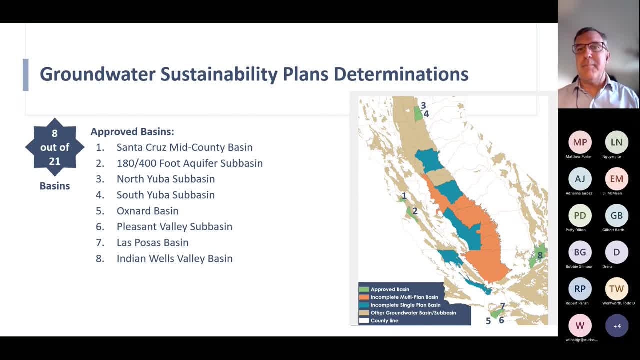 all of the groundwater sustainability plans, from all of those high and medium priority basins, including the critically overdrafted basins. again, another major milestone for for the program. people are taking this seriously and taking significant actions to to address this so they have water, water resiliency moving forward. so where we stand right now is from those basins, from those plans. 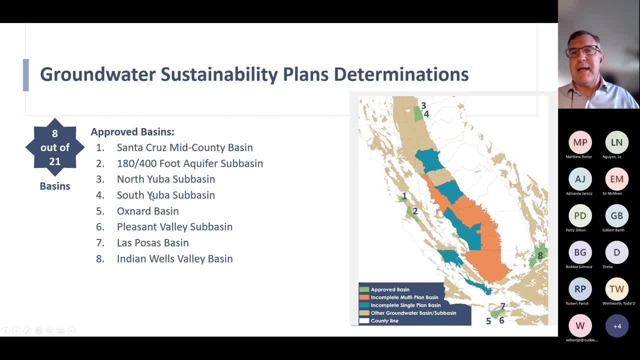 submitted. in 2020, we had eight of the 21 plans that were submitted be approved. when we approve a plan, it's not just a stamp: congratulations, move forward. more often than not, there are small deficiencies that we are asking them to correct over their implementation period. these could be: 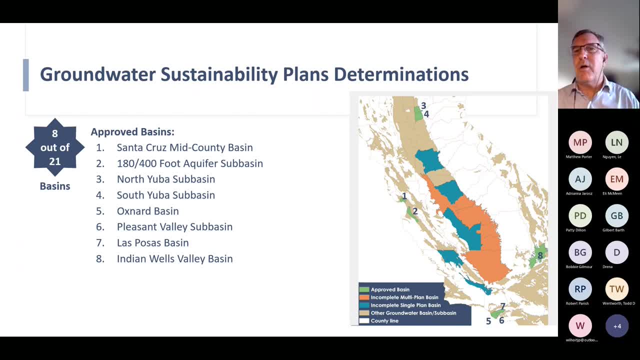 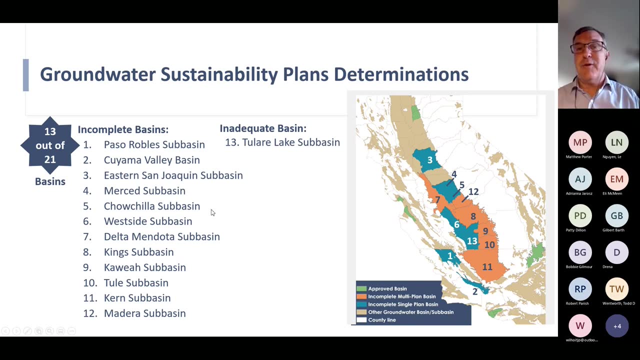 filling the filling of data gaps, addressing small, small discrepancies within their plan. so there is no perfect plan. they're going to continue to work on this and involve this throughout the 20-year implementation period. however, of these 21 plans, we also identified 13 that had significant deficiencies that needed to be addressed. SGMA allows for us to. 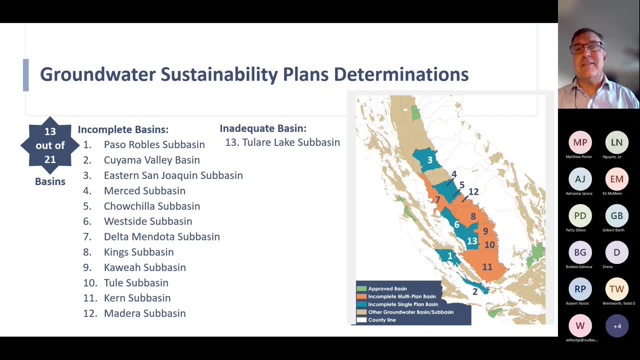 provide 180 days. it's not a lot of time- six months for these agencies to understand what the deficiency is, address the deficiency and resubmit it back to the department. so that's where we're at right now. these agencies all submitted, resubmitted, their plans. 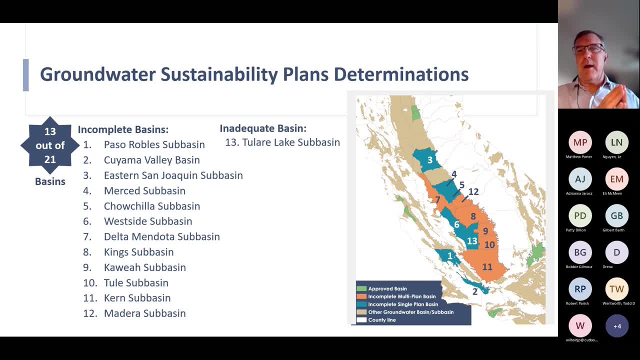 back in July of 2022 and we are about ready to start releasing the assessments for those resubmissions. so within this first quarter, we're going to start rolling out the assessments that really tell them what track they're on. are they going to be talking with the state board or are they going to continue? 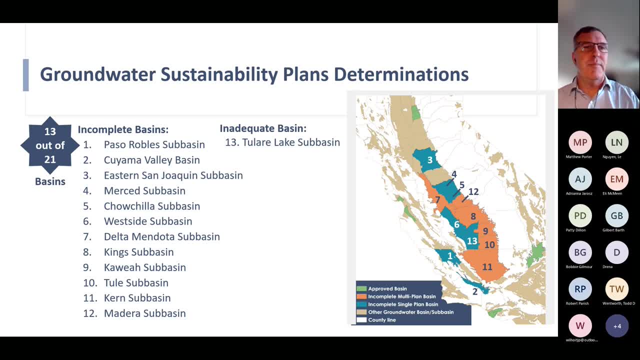 to implement their plan and address recommendations from the department. you notice there's one basin out here that was identified as inadequate and that was really an administrative issue, and they've been working with our sister agency, the backstop at the State Water Resource Control board, to rectify that and keep moving forward. remember the intent of sigma is for local control. 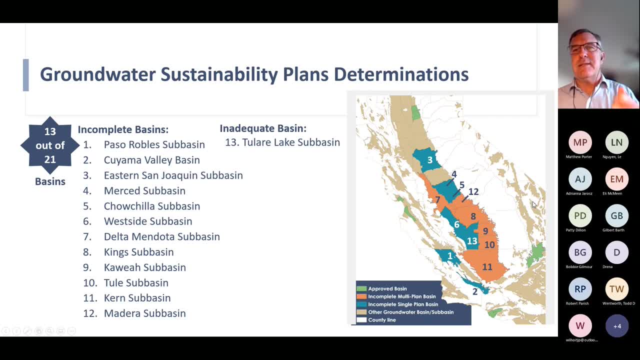 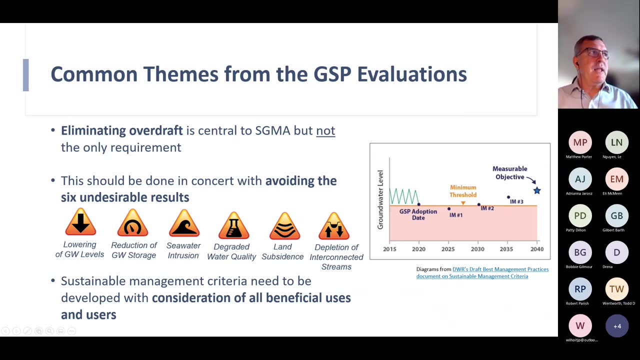 so, despite a determination of inadequacy, it is the intent of the state agencies to correct the deficiencies and get them right back into local control and local, local implementation of their plans. so some of the some of the common themes i included this slide just to help you understand. 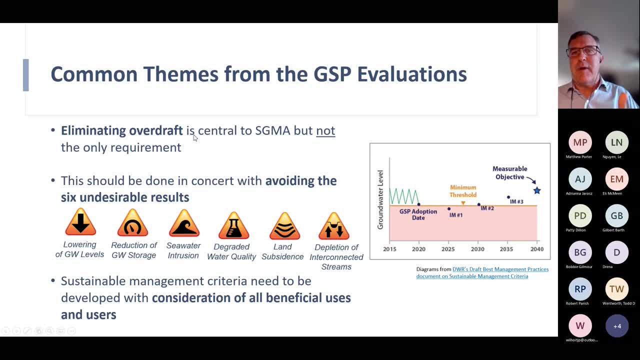 you know the big, the big ticket item is eliminating overdraft. but that's not the only thing right we? we still have to consider how the groundwater conditions. you may have eliminated overdraft but you may be operating now at a lower groundwater level. that may have an effect on. 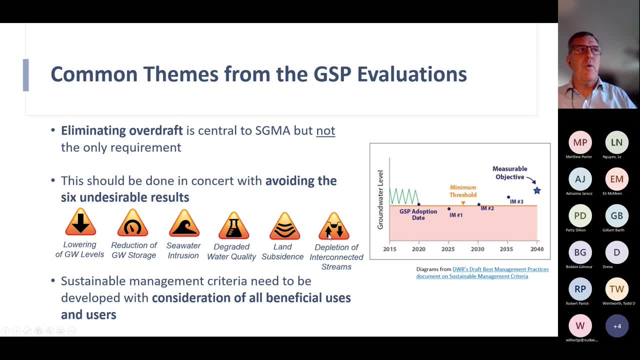 subsidence may have an effect on seawater intrusion or the depletions of interconnected surface waters. so it's a very tall order to think about one of these actions. but then how do these actions relate to one another and how does how does this play out? so we need- we need the local agencies to have some time to. 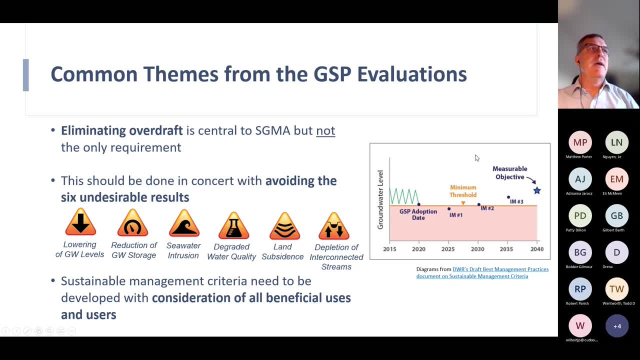 work on these things and that's why we're working with them to provide this. the graphic on the right really kind of illustrates some of those quantifiable metrics that we described, and this comes from some of our guidance documents that we put out to support local agencies in. 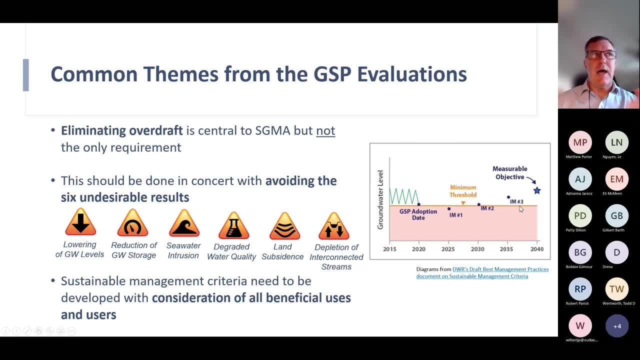 getting through this so you can see there's a minimum threshold line. you know below which bad things can happen. but one of the things i want to highlight with this graphic: you can see there is a, a dot there, im1. we also define that. they can say: we have interim milestones, so a basin may be. 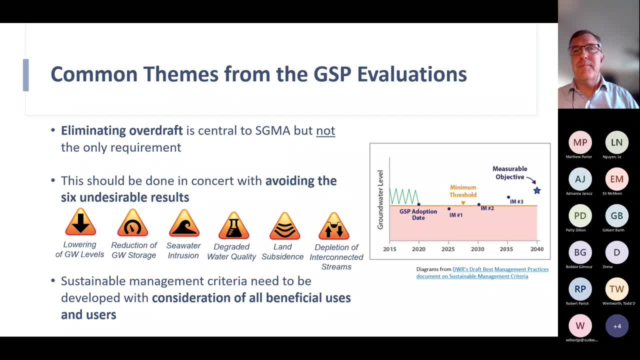 on a trajectory heading towards those undesirable results. but we recognize that they may be implementing projects to to rectify that thing. so we acknowledge that they might dip below that minimum threshold line. but then as the project gets implemented, as they add additional supply, we'll see it come out of that and start leading towards its. 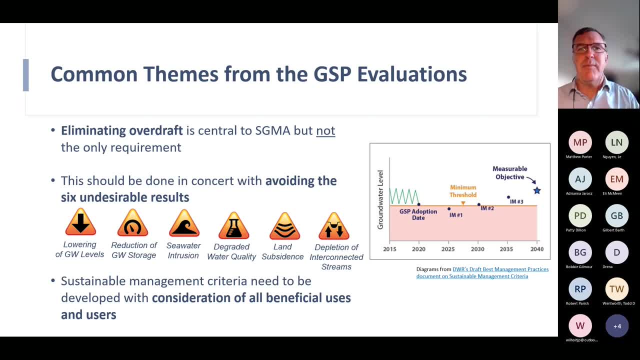 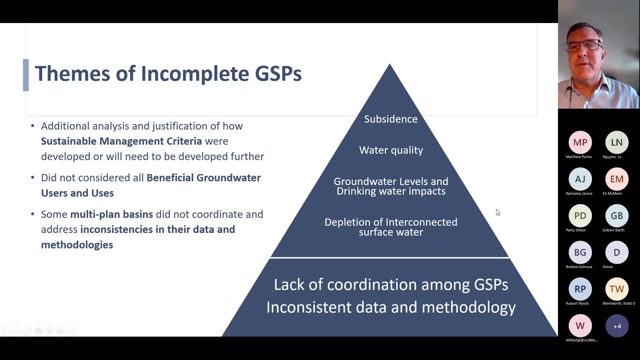 measurable objective that's. that's just one of the many pathways that that local agencies are looking to get through this, but the bottom line is it's all based upon what the impacts are to the beneficial uses and users in the basin. so what are some of the common themes that we're? 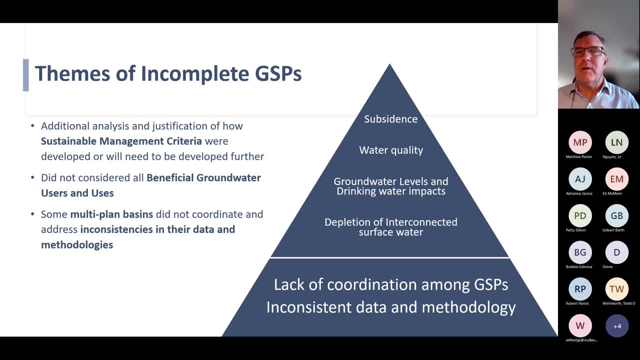 seeing in in our assessments and what's what, where the challenges lie with the groundwater sustainability plans. so i mentioned the multi-gsp, multi-groundwater sustainability plan basins. the lack of coordination is probably the most significant, even in the basins where there's single plants. it's about being coordinated, it's about bringing people together and talking through. 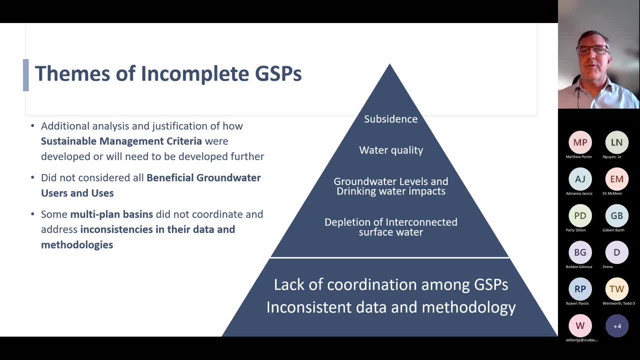 the appropriate methodologies to quantifying what the water resources are and how best to implement those. other significant challenges that we've provided comment on um are: the depletion of interconnected surface waters, groundwater level impacts- so chronic groundwater level declines, and how they affect those beneficial uses. and how they affect those beneficial uses and how they affect. 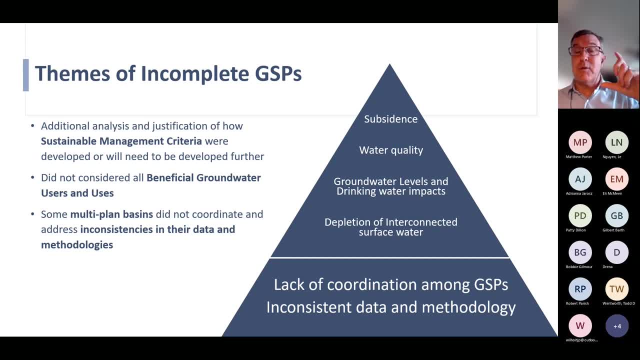 those ventures and uses. as you can imagine, domestic wells are commonly the most shallow wells, so when you drop groundwater levels, uh, pretty far, you can start to dewater those wells and we're seeing a significant impact throughout this drought that we're experiencing right now, in that 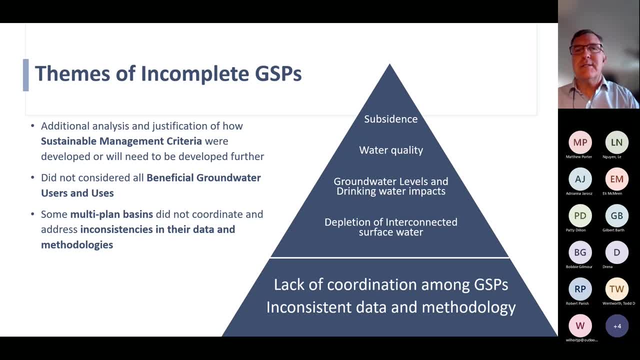 arena. water quality, including including discussions of water quality is, is important and required as part of this act. despite there being an entire another set of regulations that manage water quality, both of surface water and groundwater, people are not being able to access groundwater- groundwater within the state that that lives under the state water resource control board. 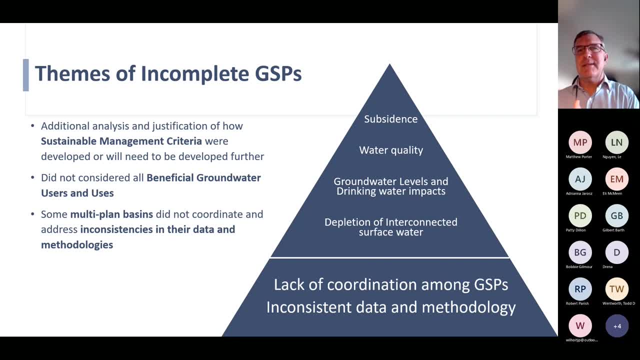 it's really acknowledgement that that program exists and understanding as to how they are going to, you know, complement those efforts and make sure that those groundwater quality conditions aren't exacerbated through the implementation of their plans. and probably the most significant one is subsidence. and if you're unaware of subsidence, subsidence is one of those conditions that 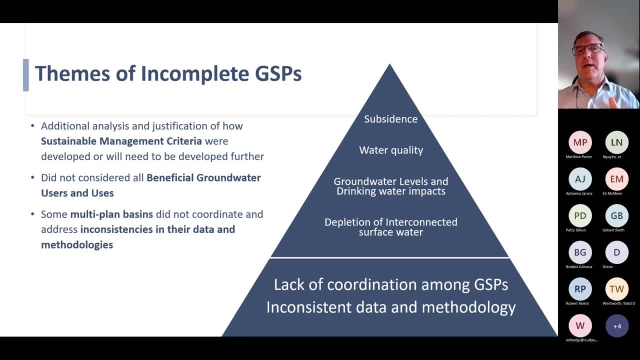 due to groundwater pumping, we are depressurizing, confining layers, the clays in these aquifers, and allowing for the collapse of those clays. when that collapse occurs, we we start to see a deflection of the land surface downward as those sediments compact. that both represents a loss of 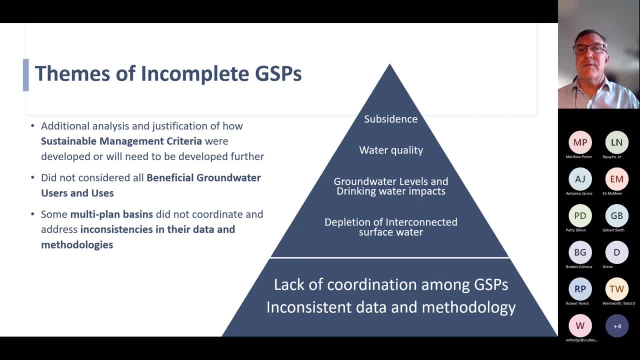 storage but also has a significant impact on the surface infrastructure that we rely upon. of note the central valley project, which is our federal water project. it runs along the east side of our san joaquin valley, the central valley. they experience some subsidence conditions in the 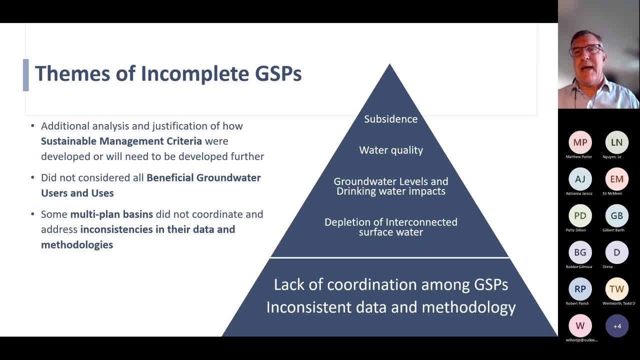 region that have resulted in a loss of capacity- conveyance capacity- of that canal of up to 60 percent. that's cutting off a huge amount of water for a lot of people in the southern end of the san joaquin valley and is really creating problems. the federal government state. 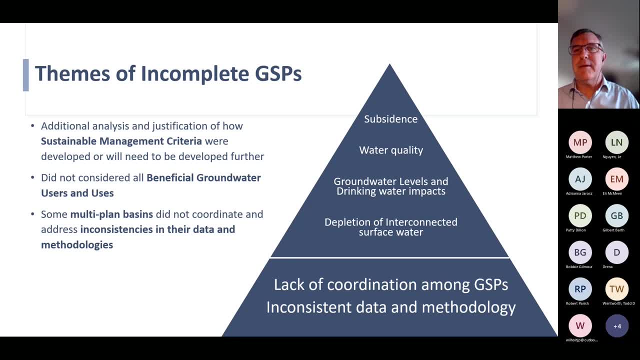 and local governments have all chipped in to repair these things, but we need to address the root cause, which is the subsidence, the over pumping of those aquifers, and that's where, that's where sigma comes in. so we're doing those simultaneously and i'll just say it's not without a lot of 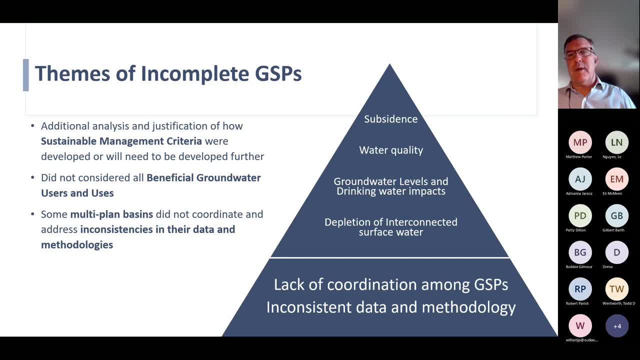 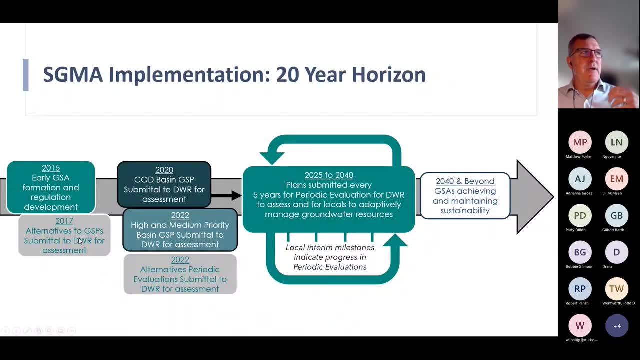 significant challenges ahead. so quickly on implementation, you know we've done all of these things i've described. we've got the law, we established gsas, we've received the first plans for all of the, all of the different categories and we're out here in implementation. so once the local 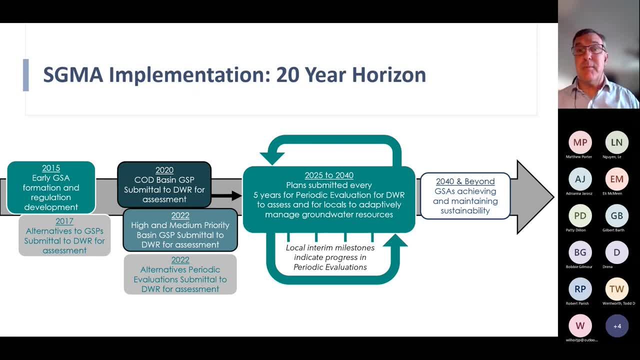 agencies have locally adopted these plans. they are in implementation mode. our job is just to say whether or not it's compliant with the act. they still have a plan that is very pertinent to their basin. it may not quite pencil out, but it's something that they're going to work on over the 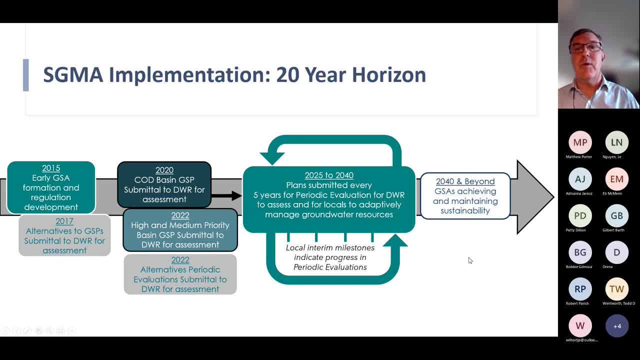 next 20 years. they're all required to reach their sustainability goals by 2040 or 2042, depending upon what they're starting to do, so we're going to have to work on that, and we're going to have to work on that, and we're going to have to. 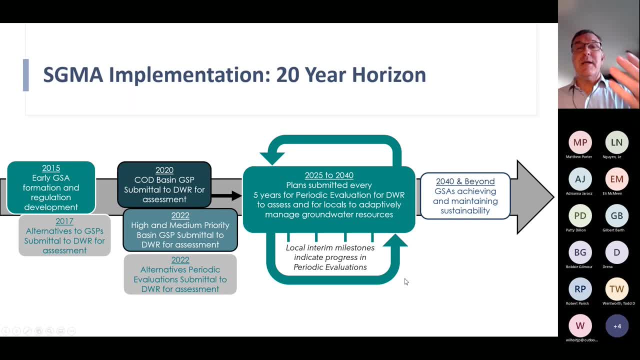 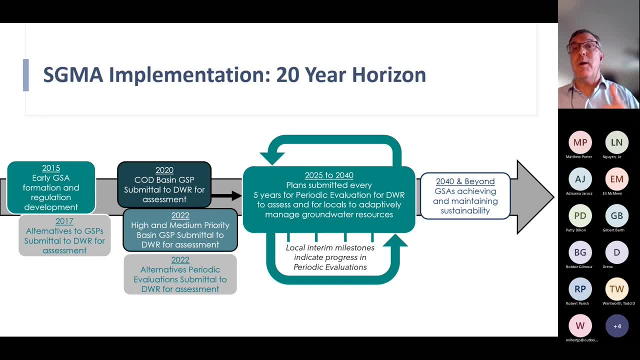 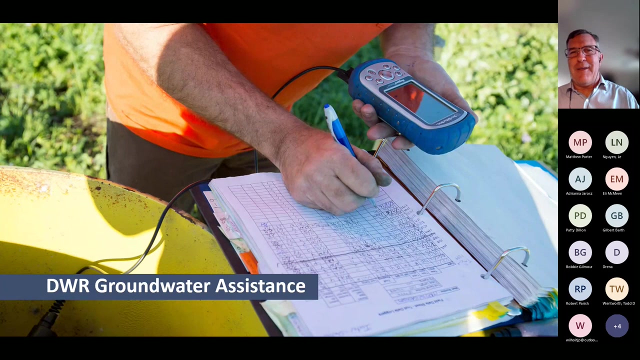 basin annually. they are also required to report quantitative values for the cumulative groundwater extraction and, ideally, reporting on implementation progress. how are they implementing their projects and management actions to support their plan? So that's the regulatory aspects of what DWR is doing. I find this to be the best part. 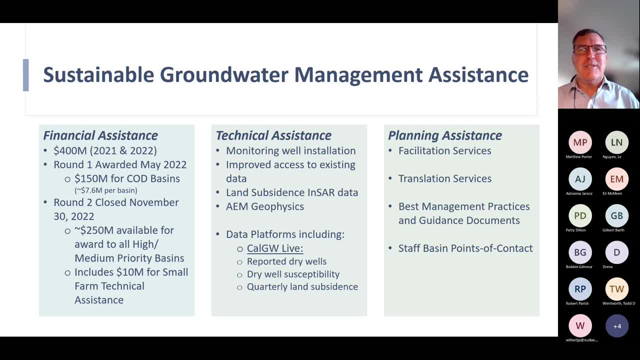 What kind of assistance are we providing? One of the things that I've really appreciated about joining the Department of Water Resources is really the vast volumes of data that they had already, the willingness to collect more data and, most importantly, making all of that data readily accessible. So I'll share some websites with you where you can see some. 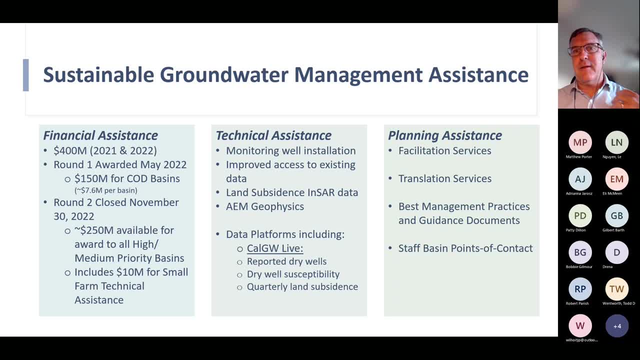 of the volumes of data that we've pulled together to make SGMA function, allow local agencies to be well-informed as they're making critical decisions. But in general, our assistance program falls into three buckets: Financial assistance: We've rolled out over $400 million. 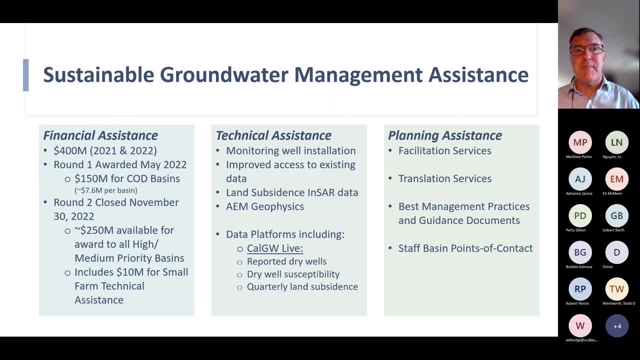 to these local agencies to develop plans and develop projects and management actions and get them started. Technical assistance: We've been physically out there installing new monitoring wells for them. We've been revising existing data sets, like our well-logged data sets, making them not only more accessible, 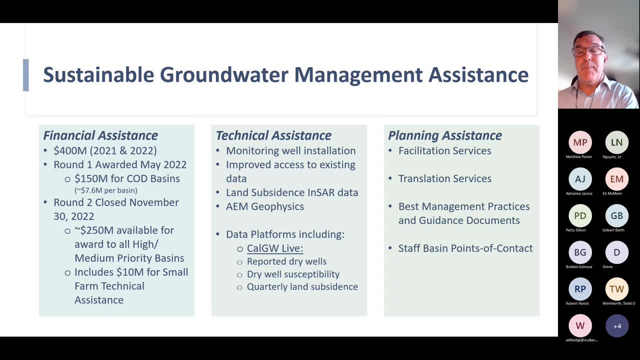 but digitizing them so that they can be easily adapted and input into numerical models or other uses. electronic uses: We've been collecting land subsidence data- This is NSAR data, remote sensed data set that evaluates the land surface- And we've been advancing aerial electromagnetic 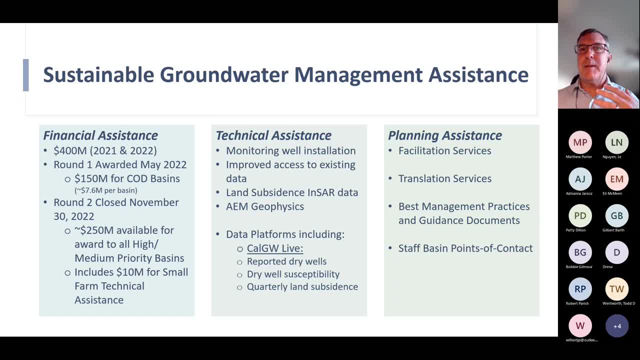 geophysics to help characterize these basins further, to tell people where are we going to be seeing the greatest proponents of coarse-grained sediments versus fine-grained sediments, so that they can make informed decisions as they're implementing projects to enhance supply. 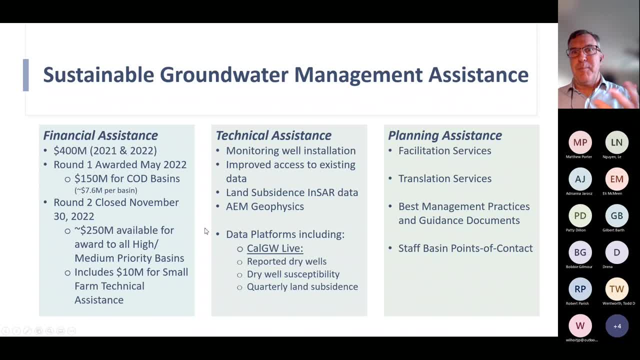 like recharge projects. We've also provided a number of platforms to access these data. So one of our flagships is the Cal Groundwater Live webpage. You can get on there and see kind of the current state of conditions within our groundwater systems. All of our data is funneled back through there. 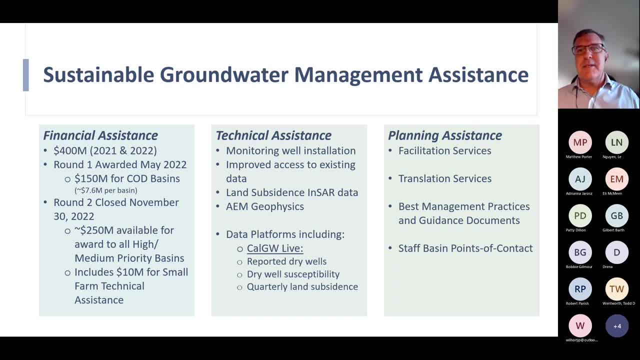 it's coming from these GSPs, So we're still building some of these things. They're going to be continuing works in progress. We'll add new bells and whistles as we go, But if you're so curious, I'll share these links and you can browse around. 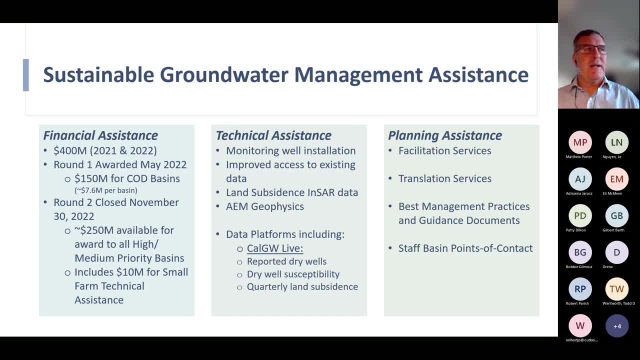 We also have the SGMA Data Viewer, which is a parallel product. Cal Groundwater Live is a little more focused on public entities- folks wanting to understand what's going on in their basin, And the SGMA Data Viewer is really focused a little bit more on the technical. 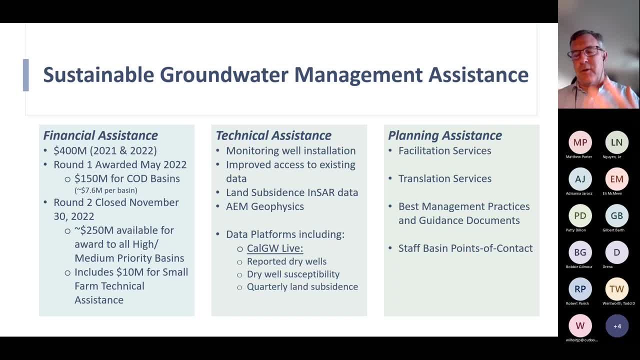 practitioners. We're really looking to access the data. It's a great map, but all of these datasets are made available through our California Natural Resources Agency's open data platform And this is a big, big push that SGMA has been leading the charge on a number of fronts. 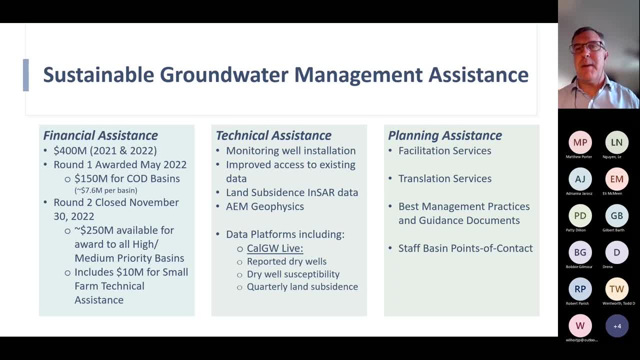 and providing all of our data out there in a very transparent manner, And that's one of our big driving mantras here is that we want SGMA to be transparent. There isn't going to be any hidden messages or backroom discussions. This is all happening out in real-time And it's a little uneasy for most folks. 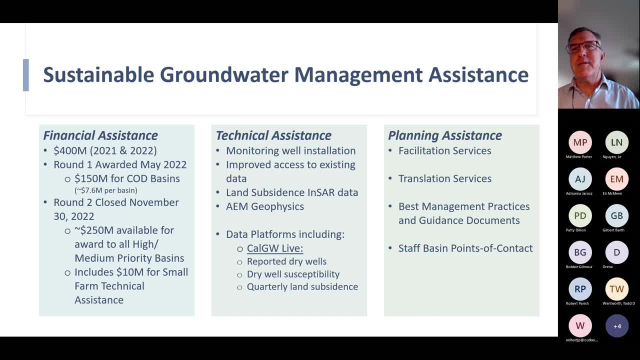 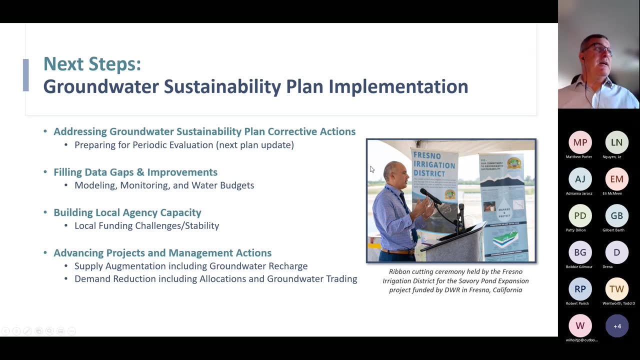 involved with this, but it's having an effect and people appreciate the openness and conversations and now have a greater understanding as to how the decisions are being made in some of these basins. So where are we now? The next steps? through our implementation, We're really supporting. 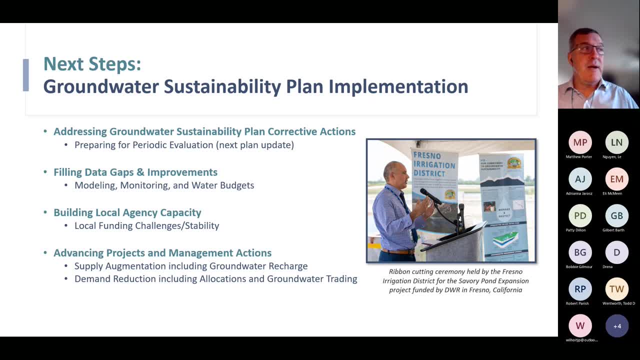 local agencies in addressing their data gaps and addressing their issues, And so this is our strategy. We're really recognized as the best if it's something that's going to be a and addressing their corrective actions. we're providing a lot of data and and support through 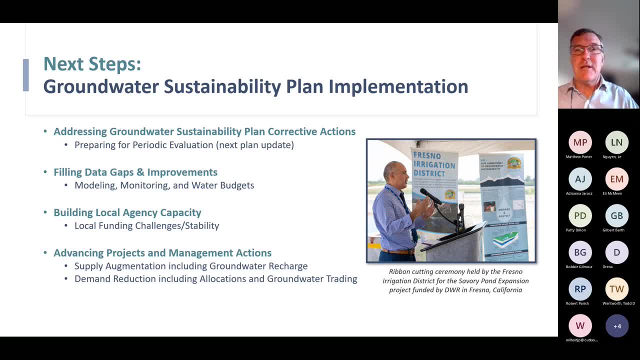 our regional offices. we're providing that funding, getting projects off off the ground, getting new recharge efforts going on um. we're also building that local capacity. we're trying to provide support to these groundwater sustainability agencies because they're now faced with implementing what are quite expensive projects to achieve. so they're having to go out and and we 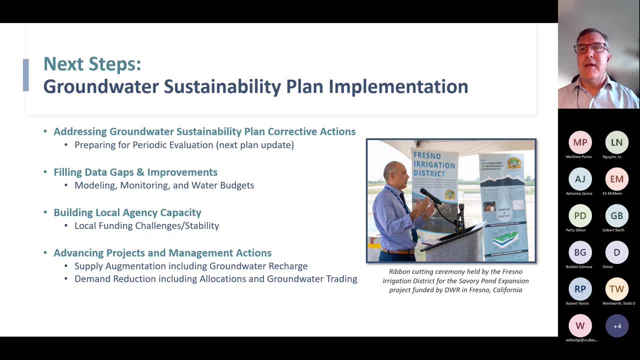 have a function here: a law within the state that requires any new fee or tax that needs to go to a public vote, and it's very challenging to explain to somebody. we need x number of million dollars to implement this recharge project and you should vote for this, so we have a large educational 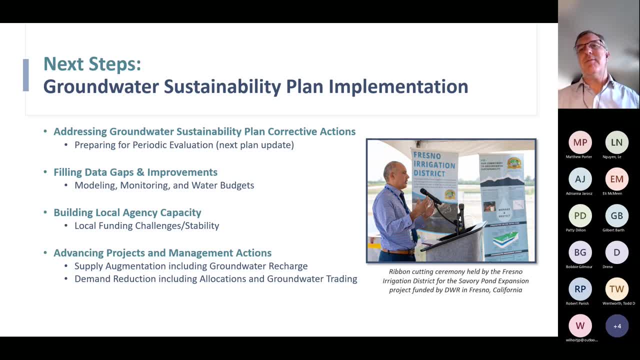 campaign going. we're trying to help locals understand where their water is coming from, why, why it's important for the gsas to receive the funding they need to implement the plan. so it's a real challenge from an educational standpoint as well. so, oops, we're. we're not only, you know, thinking within our 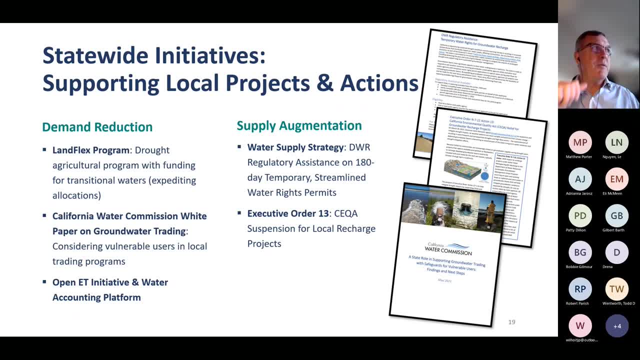 box of sigma, but we're broadening this out and making sure that people understand. you know what, what, what poss, what possible support structures are out there. so one in particular where we've put out there- just actually two days ago we've released the landflex program. 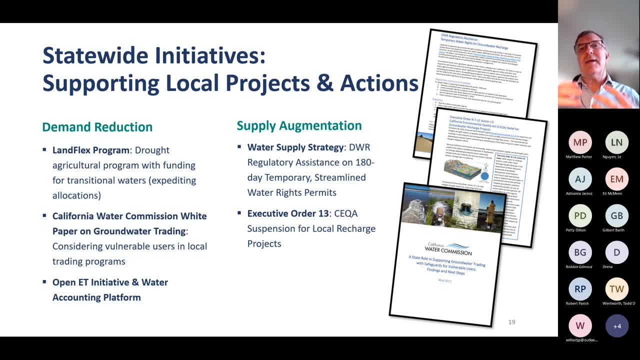 this is really a following type of program that is targeted at addressing where agricultural lands sit adjacent to disadvantaged communities who are experiencing depletions of their drinking water supplies. so we're talking about taking those agricultural lands out of practice, stopping the pumping from those wells that may be affecting the drinking water supply for those. 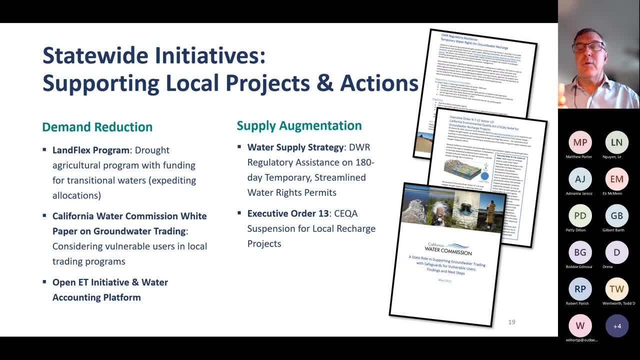 disadvantaged communities and paying for those local, those local growers, to transition to what is a sustainable groundwater management allocation that has been provided to them for the acreage that they have. there's a lot of a lot of cuts coming for a lot of these basins. they've been 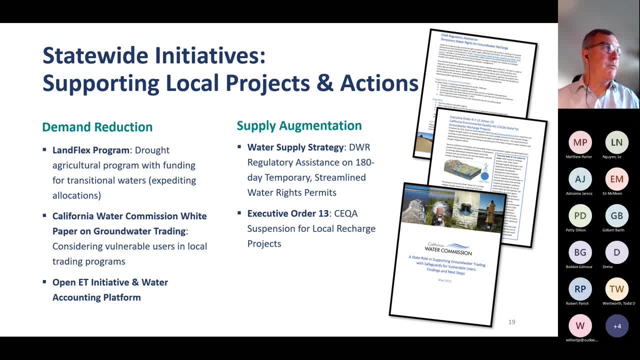 significantly overdrafted for a long time. so a big program that we're rolling out. currently we're also advancing concepts about groundwater trading- how can we trade our allocations within these basins- and we're we're helping local agencies prop up accounting platforms so that they can 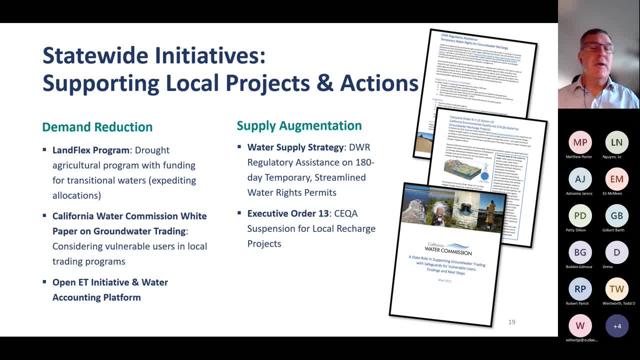 accurately and transparently conduct these trades of these groundwaters. and- and that includes the- the use of open et- and i don't know if you've heard about open et, but it is a an open source software package being developed by environmental defense fund and um and others. uh, that really. 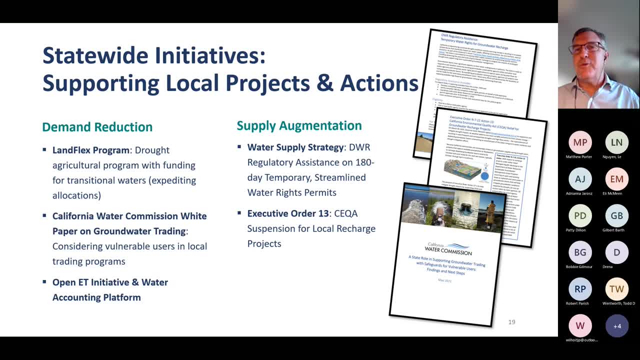 is a remote sense based water use estimate. it's a model um, but it helps kind of level the playing field about. i grow this type of crop. it uses x amount of water. that type of crop should use similar amounts of water but climatic changes, uh, or climatic conditions, affect that that volume. 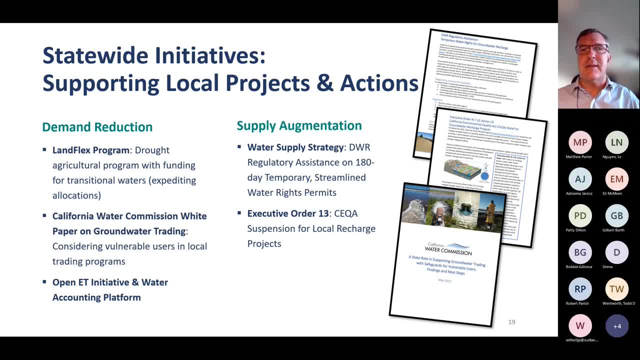 so this estimating tool is useful at least at leveling the the playing field for people to have conversations about how water gets traded and accounted for within these basins and supply augmentation functions. you know we've we've had a number of uh recent water supply strategy paper that was released that really directed our department at finding ways. 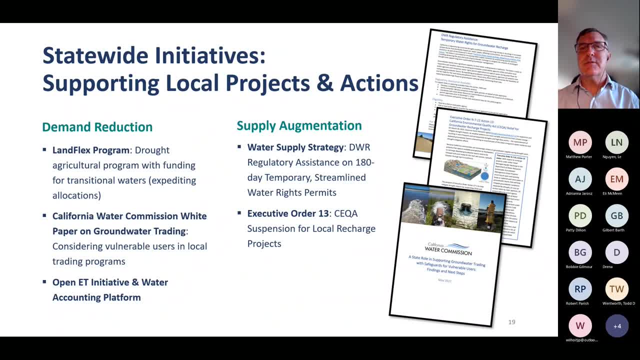 to expedite the permitting process for conducting recharge. so i've been involved with that quite closely and we are- we are working hard to make sure that we're capturing those high flows when they're present and spreading them out on our land surface, allowing them to infiltrate. 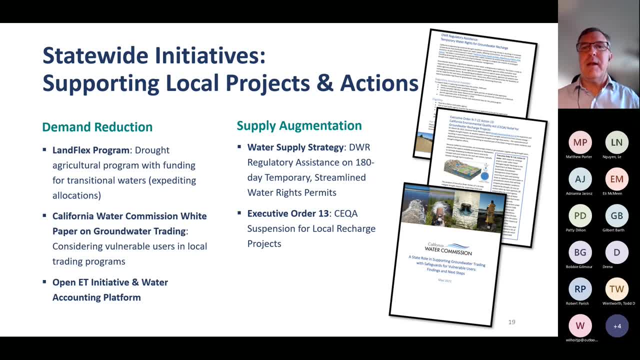 and recharge our groundwater basins, but we're coming out of a legacy- legacy um period- where groundwater has has hasn't been managed in this way, and so we have a lot of rules and regulations intended to prevent the abuse of of some of these water resources, and so we're finding new pathways. 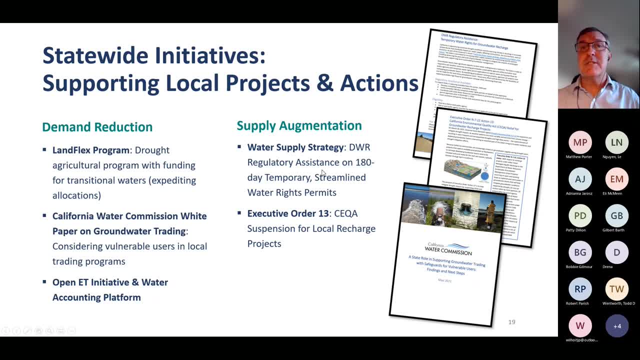 and expediting those so that the local agencies and growers can divert waters and get them onto the ground when those waters are available. uh, i'm sure you've seen the the latest news. you know: california's been in a three-year drought and we get hit with three weeks of storms. 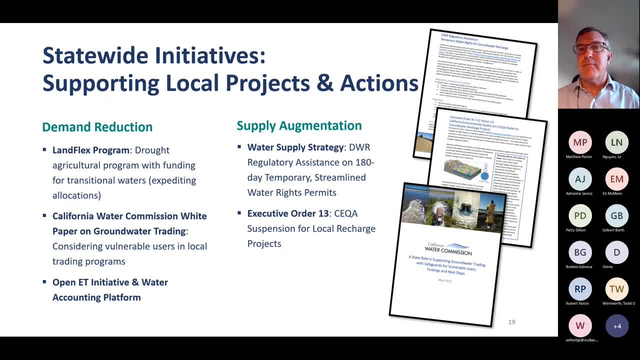 that drop tremendous amounts of water on us, almost like washington, but it's um coming fast and furious and maybe too much to manage, and so we're trying to find ways to peel those off and store them more effectively. and then, um, we're also leveraging executive orders. 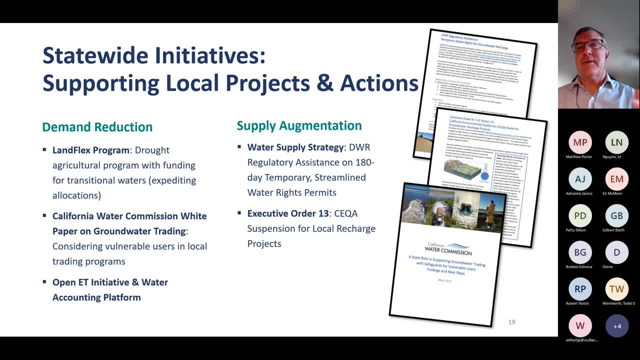 from our governor to allow us to move and act on some of these recharge projects that are we're- you know, in our mind- low-hanging fruit. let's get water out of our rivers. let's get water. get water out on our agricultural lands or open and working lands where there isn't concern. 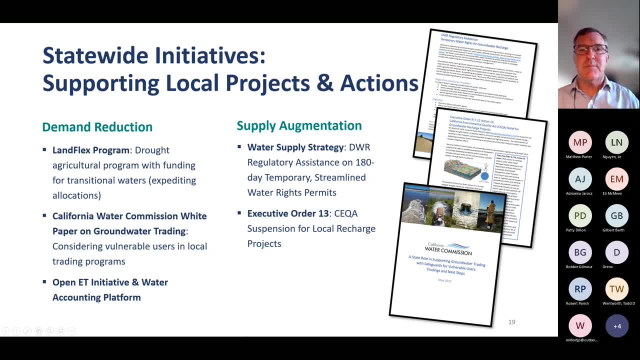 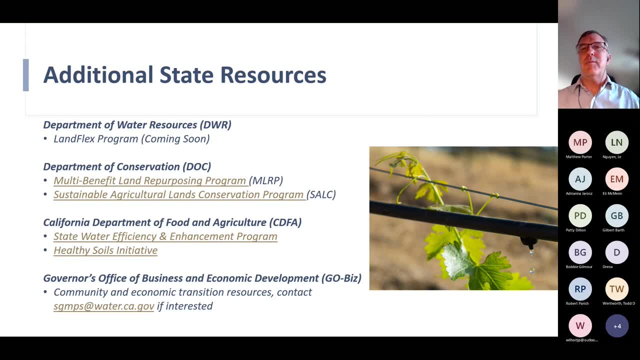 for water quality impacts and get those functioning as recharge properties to the greatest extent possible. So, beyond what the department is doing, we also are reaching out to our sister agencies across the board, throughout the state, recognizing that some transition of agricultural lands will be necessary. 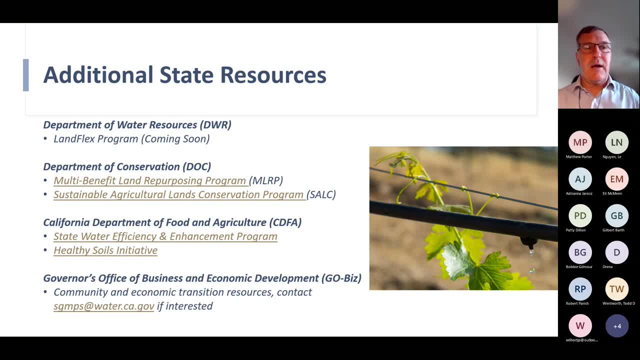 So we've engaged with our Department of Conservation, our Department of Food and Agriculture, as well as our governor's Office of Business and Economic Development, recognizing that some transition of our workforce may be necessary to accommodate changes in our land use practices. So a lot of moving parts here and we are at the starting gate, still on SGMA. 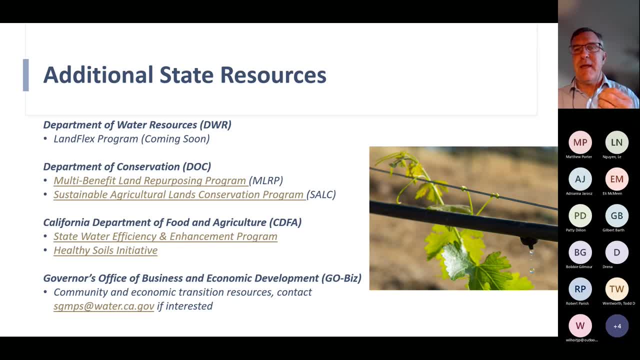 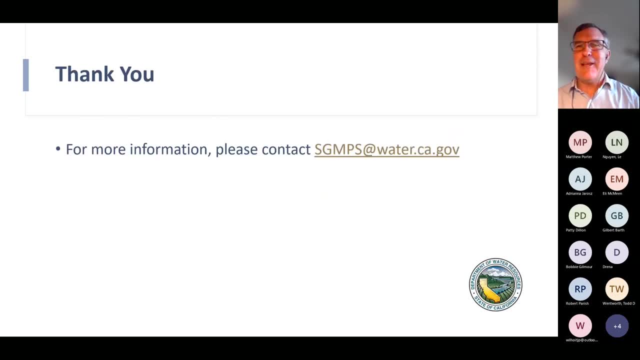 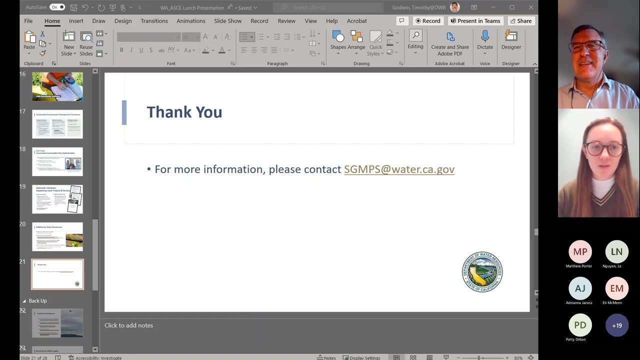 So things are going to take a little bit of time to take effect, but they are acting now and I think we're heading in the right direction. So I'm going to stop there and love to engage in Questions and answers and have a conversation about what's going on with SGMA. 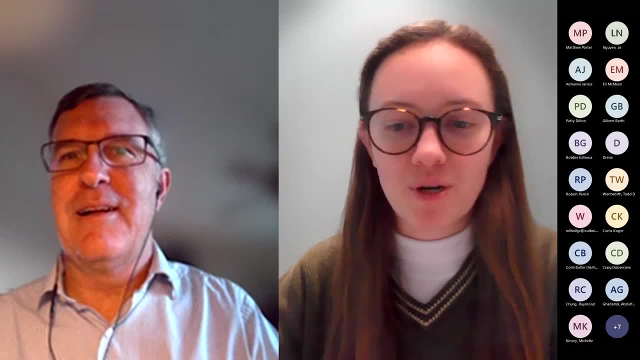 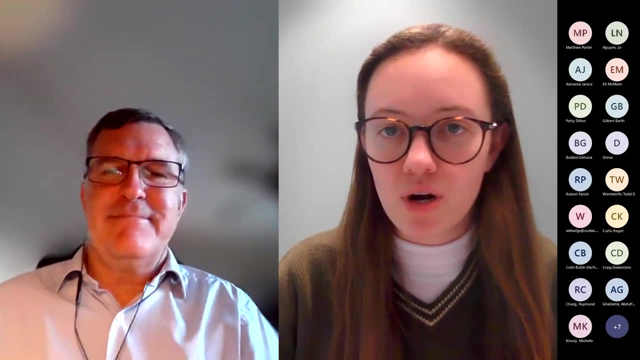 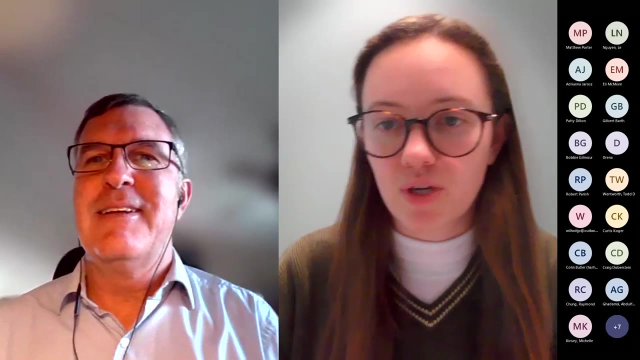 Thank you so much, Tim, for that wonderful presentation. I guess either feel free to put comments or questions in the chat or raise your hand and you can ask, or, using the reactions function, raise your hand and then we can get those questions going. 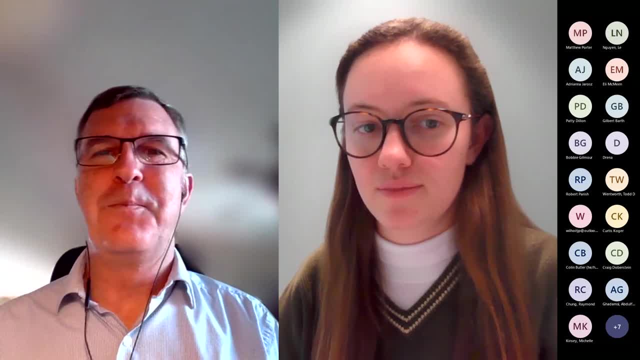 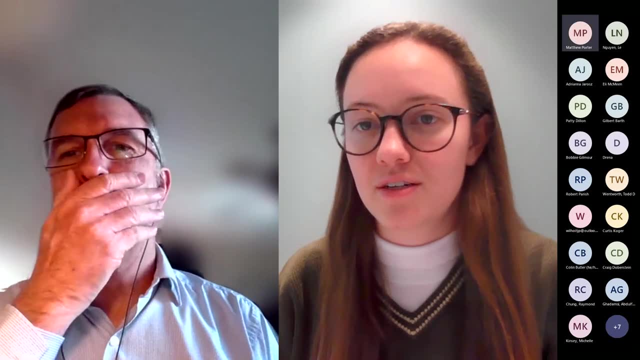 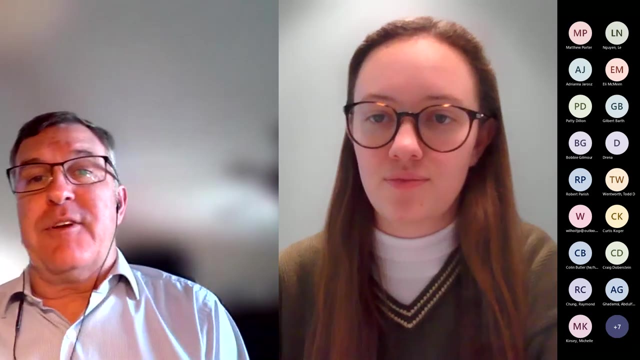 Do you think that five year updates are frequent enough, or would you like to see them happen more frequently, especially in this earlier phase? Yeah, that's a great question. You know five year interval, that was defined in the legislation and it seems to be a pretty 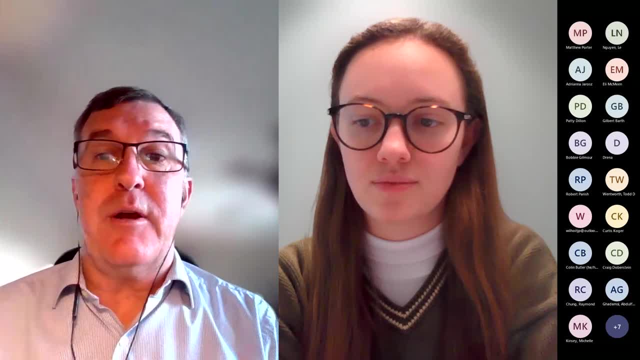 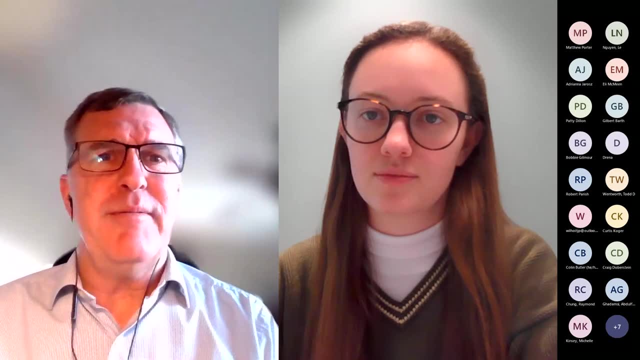 reasonable time frame for people to redress their plans. Some of these plans Are In the process of a couple thousand pages. so these aren't, these aren't small, brief levels of effort that local agencies are having to go through. You know it. 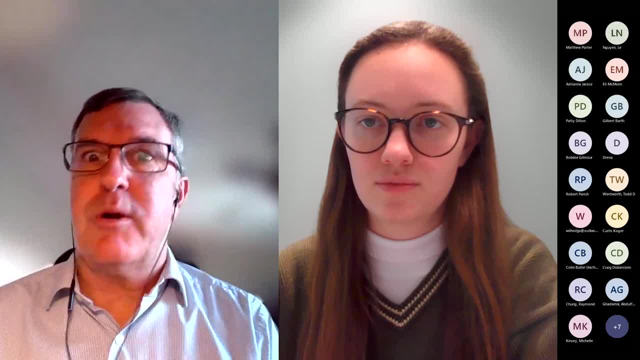 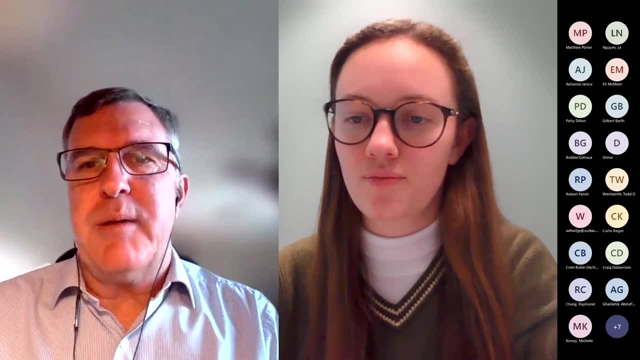 The department has up to two years to review these things and we're finding that that's pretty short as well. I mean, these are complex plans, These are large areas in many instances, So the five year intervals probably appropriate, but where we really need to go is is how we 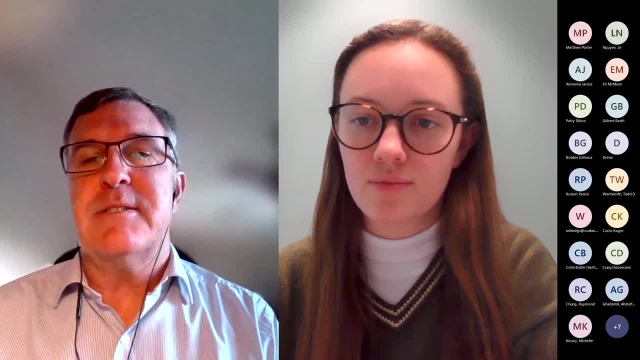 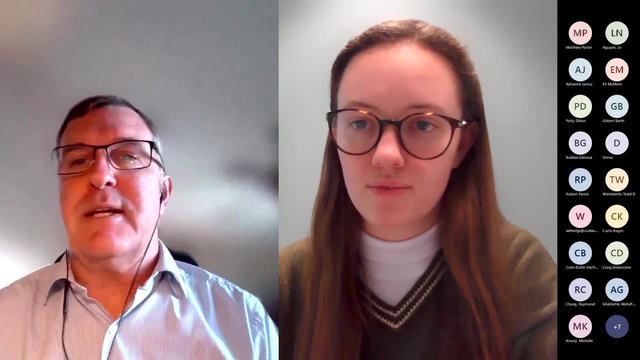 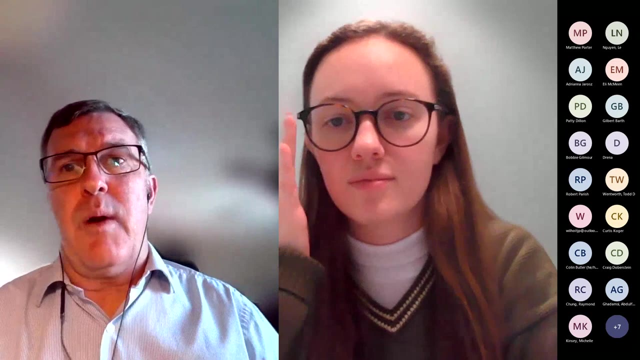 embrace on an annual basis, Small changes. engage with local agencies, Help them address. You know the changes that they're seeing. You know climate change is a significant part of this planning process, which is also unique to many of our many regulatory programs. 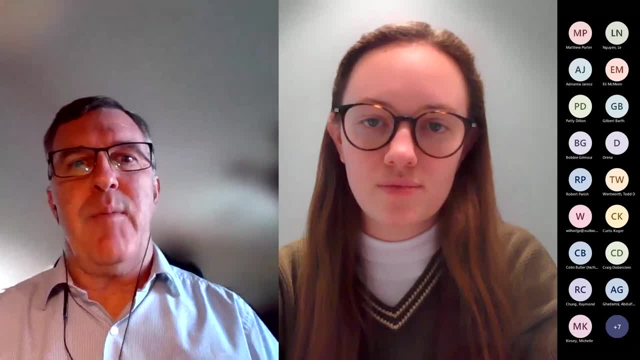 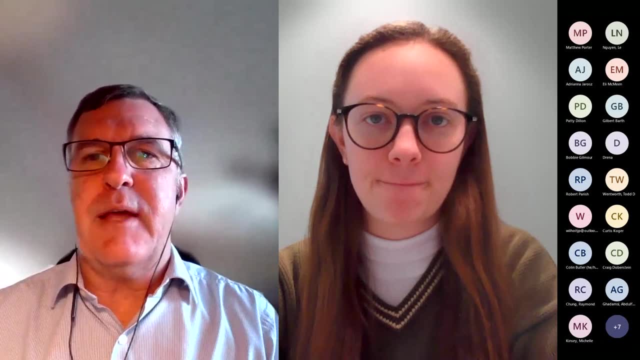 We're asking them to project out 50 years and to describe how they foresee the climate change affecting their plan. That's pretty tall order for for many of these agencies. so That's going to evolve and I think the five year time frame can start to capture some. 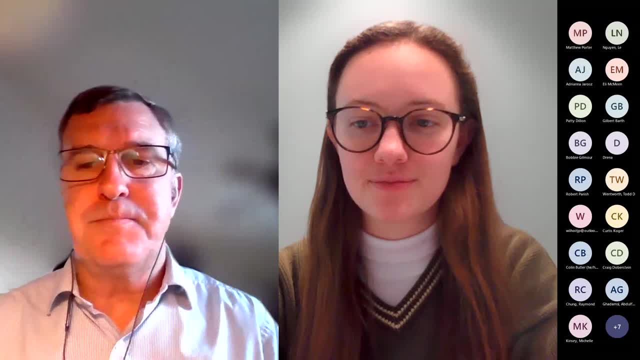 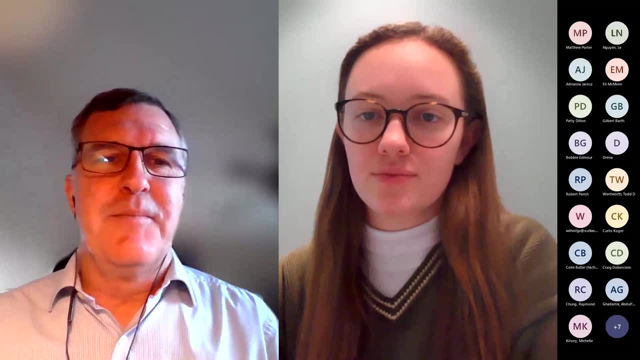 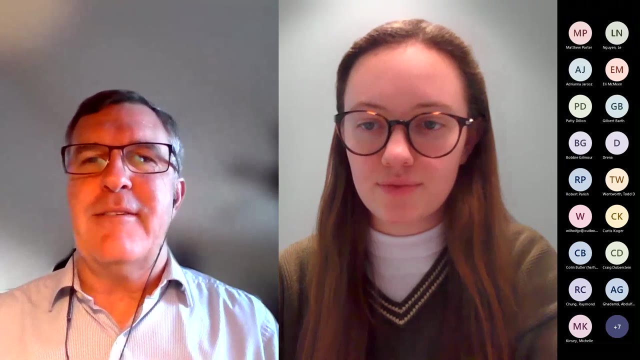 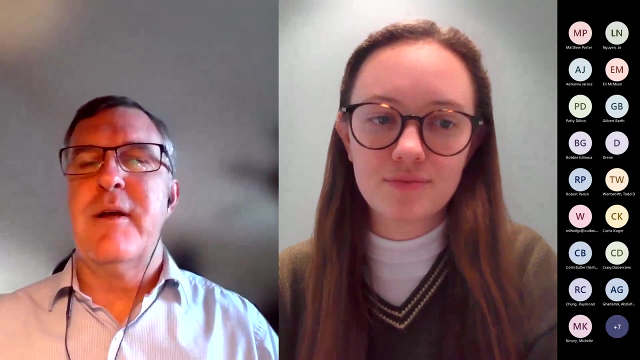 of those, Those changes, Thank you. So I think one of the one of the stark contrasts that I've I've learned in working with state of Oregon, state of Washington, looking at how they differ, is is just how the water rights are administered.